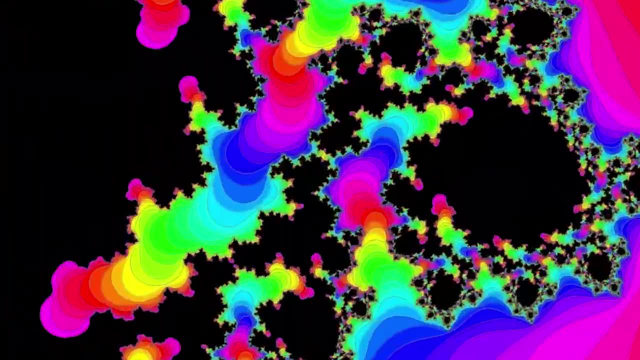 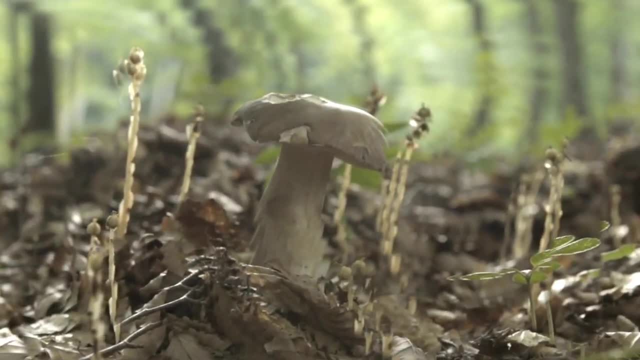 effects included in the template. It's got all kinds of psychedelic and mesmerizing animations and effects for your footage And all of the effects can be customized. So I'll put a link in the description so you can go check that out. But let's get started with how to make these. 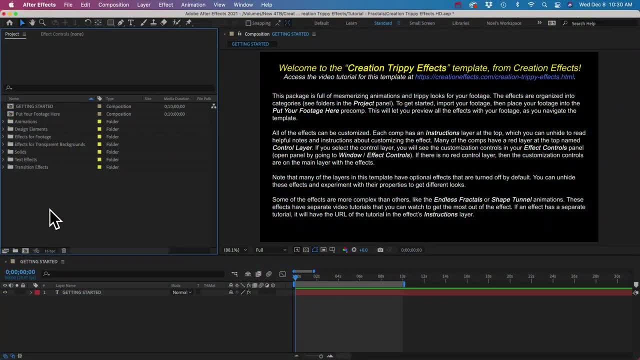 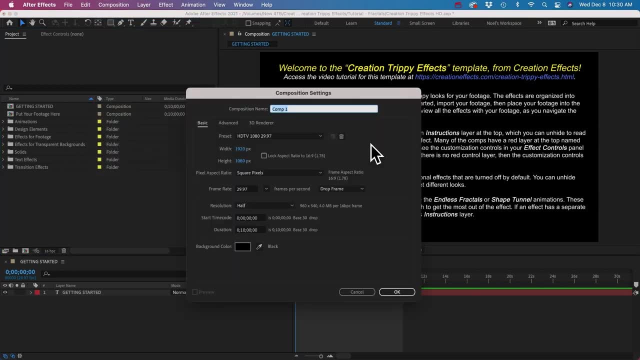 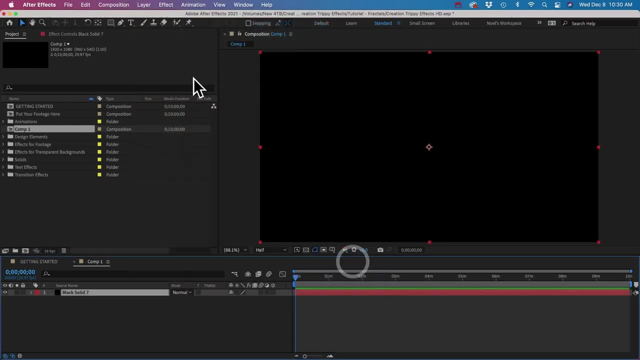 endless fractals using the template. So let's take a look at the fractal effect and we'll see why it's so useless as it is. I'm going to create a new composition and we'll make it HD and I'll add a new solid layer And I'll add the fractal effect, And then I'll add the fractal effect. 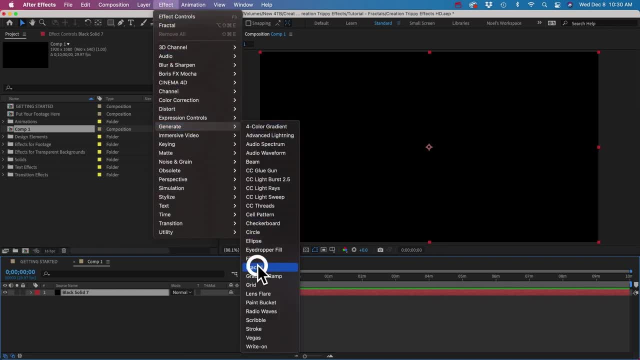 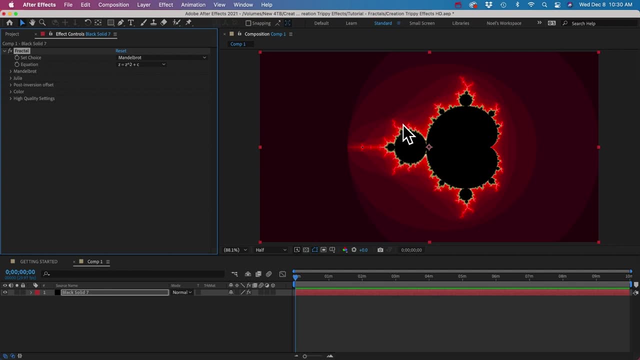 Which you can find in the generate section. So I've been trying to figure this effect out for years, because when you first apply it, you've got this kind of cool pattern, but it's not obvious what you're supposed to do with it. You can get some different patterns and you can play with. 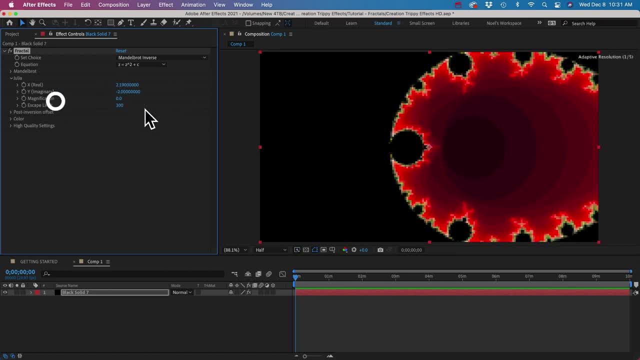 these controls, and a lot of them don't even seem to do anything. So it's really confusing, and I know I'm not the only one. I searched for a long time on the internet and I just couldn't find anyone that had found any practical application for this effect at all. 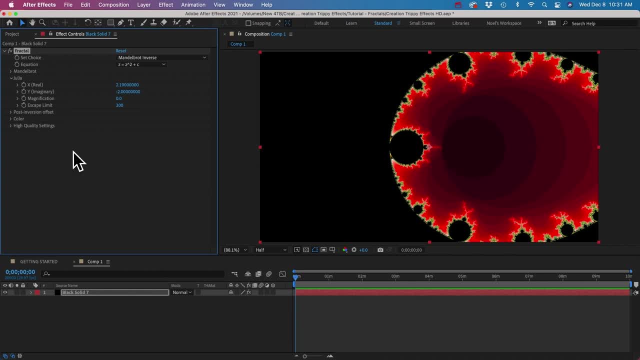 Because no one can figure it out, I think. But this latest time that I played with it, I spent enough time with it and I discovered that it's really an amazing effect. It just has terrible controls. It's not intuitive and you really can't do much with it. with 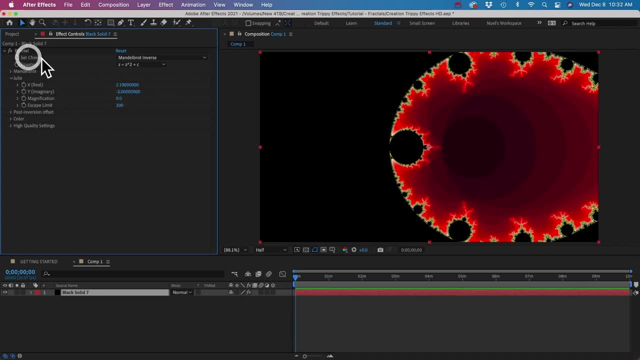 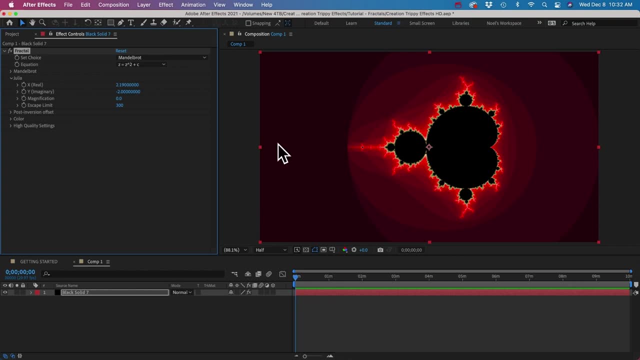 the controls as they are. First of all, this is set to Mandelbrot by default, which doesn't change anything, So I'm just going to go ahead and do that, And then I'm going to go ahead and change it. The pattern will always look like this If you set it to Julia or Julia inverse. 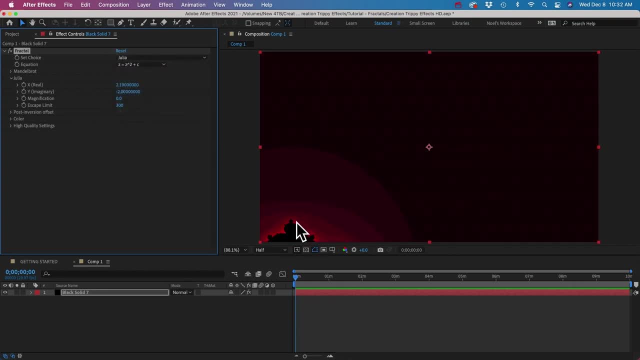 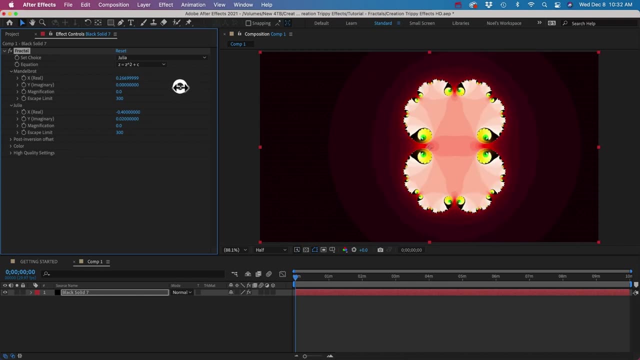 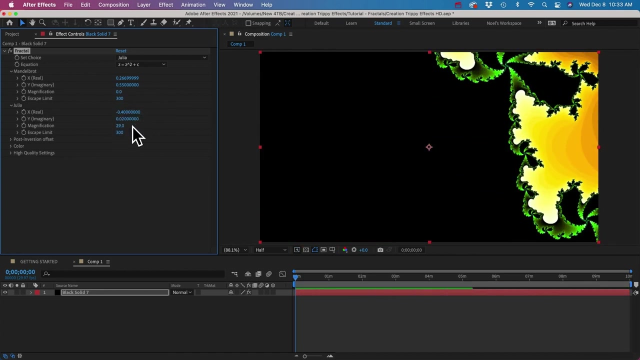 that's where the fun really begins, because you can change the shape. So you can move it around like this and you can change the shape And you can zoom in. But here's the problem. Now that I'm zoomed in, you can see I've got the magnification set to 29.. If I 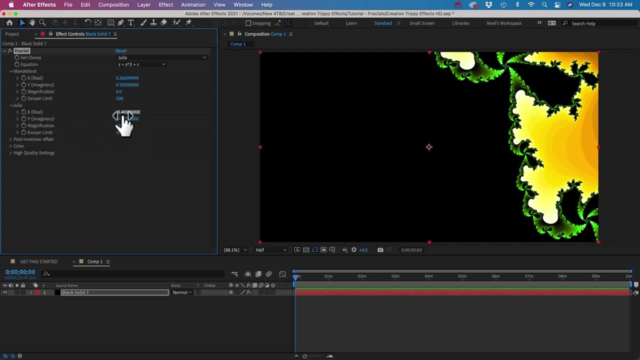 change the position of this pattern using these controls. you can see that pattern just jumps right off the frame. Once you're zoomed in, these position controls become very sensitive, So you would actually have to enter in a very long decimal number in order to get any precise. 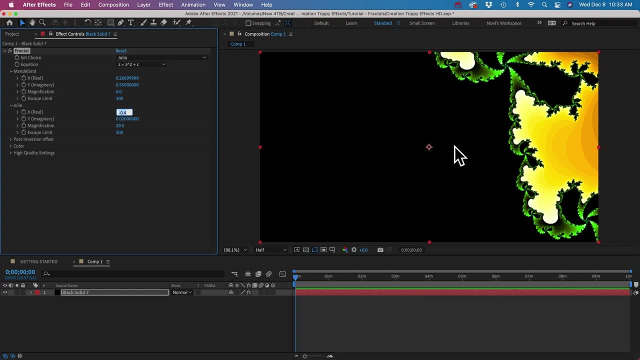 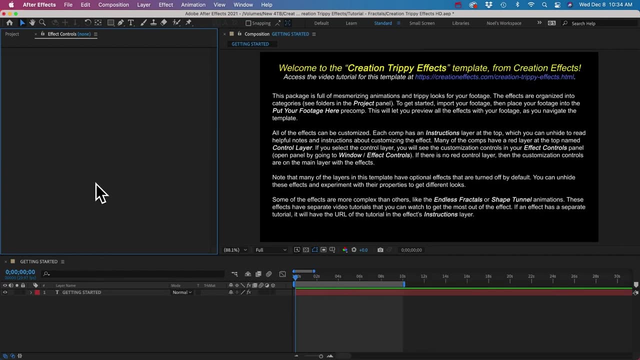 position change in here. It would be really hard and it would take forever And it would make those kinds of animations where you zoom in forever just impossible. So with this effect I've attempted to correct that problem and just make some new controls that are more user-friendly. 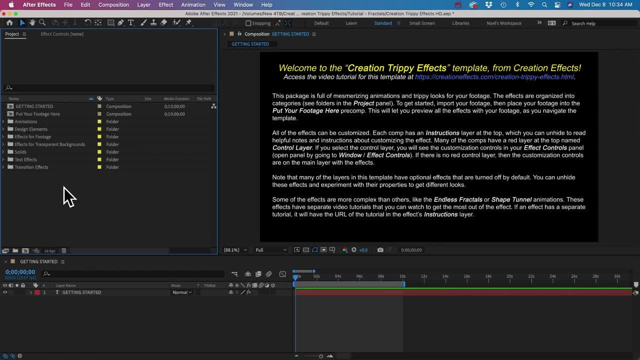 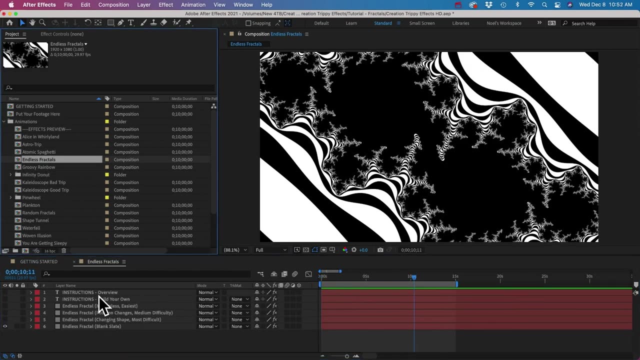 So let's take a look at that. I've got my Creation Trippy Effects template open here and the endless fractals are located in this animations folder here. Just go to endless fractals and I'll open that up. So in this comp we've got a couple different instructions layers. 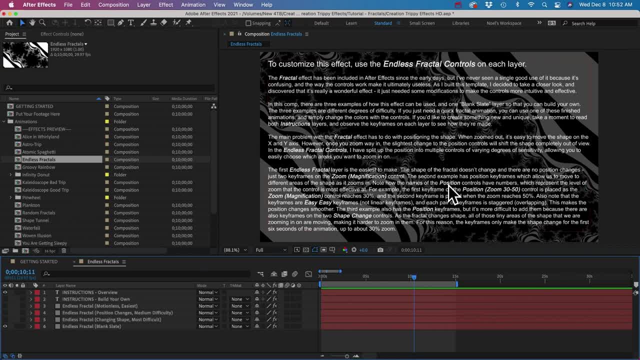 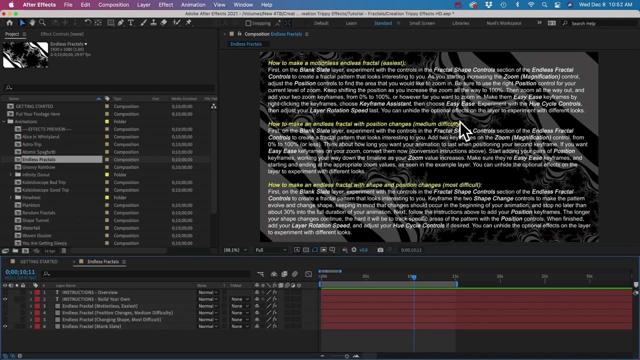 at the top. And this first one just kind of gives an overview of the effect, And the second one: you can see that the animation is now in the animation folder. So you can see that the animation has instructions for making three different kinds of fractal animations with different degrees of. 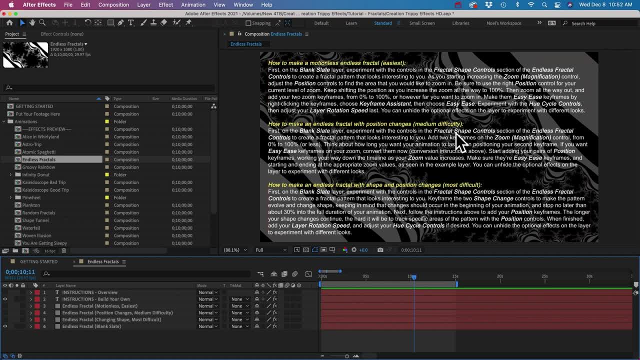 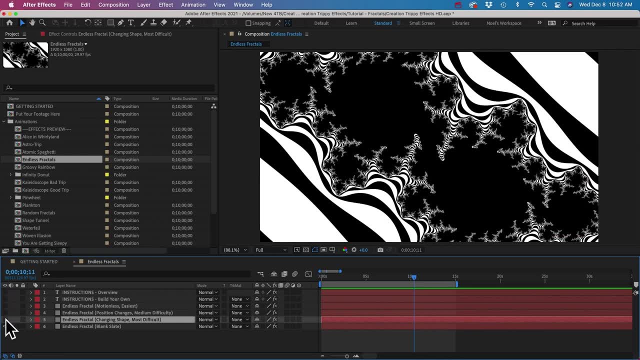 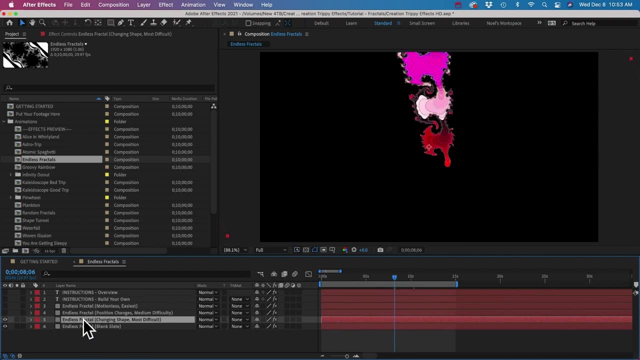 difficulty. So we've got the easiest, the medium difficulty and most difficult, And you can see examples of each of these here on these three layers. If I select a layer and hit the U key, that will reveal the keyframes that I added to make this animation And. 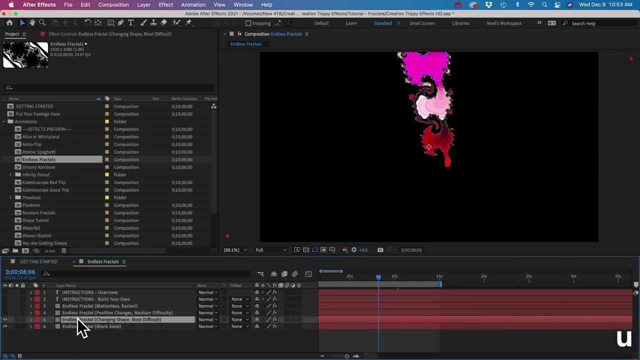 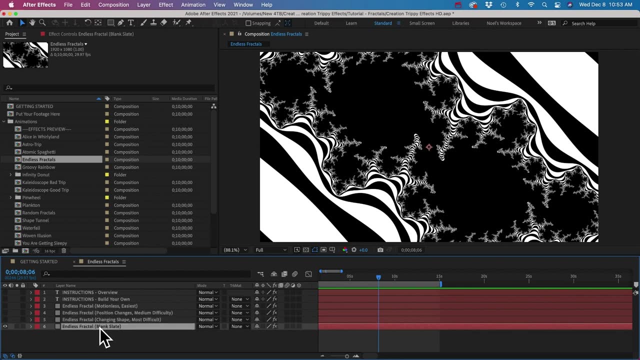 you could customize these if you want, but these are more here just to see as an example. If you're going to create your own animation, I recommend you use this last one, Blank Slate, And to see the customization controls, you just select the layer and then go to your. 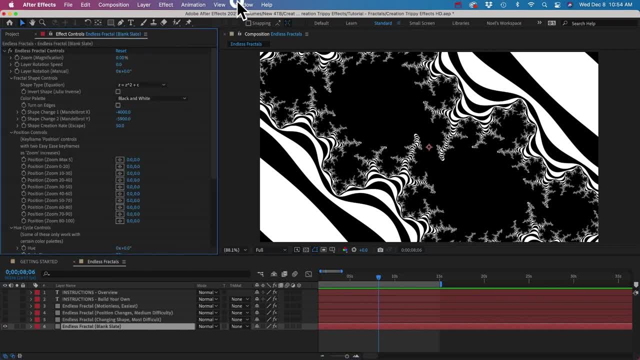 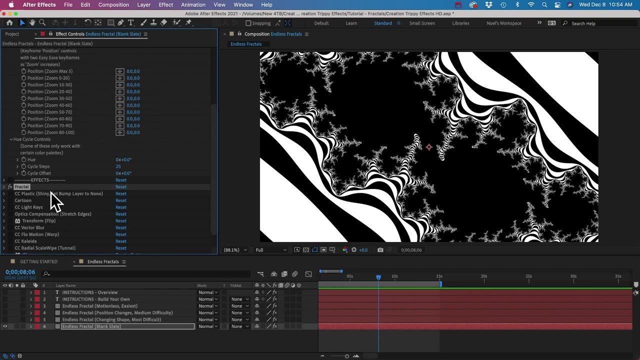 Effect Controls panel up here, And if you don't see this panel, just go to Window and choose Effect Controls. You can see all of our customization controls here, followed by the fractal effect and then a bunch of optional effects which are turned off, and I'll show you. 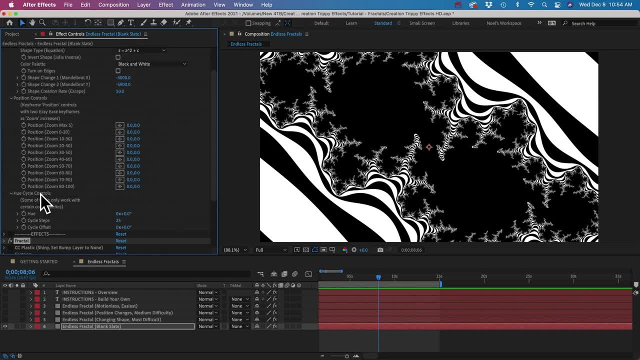 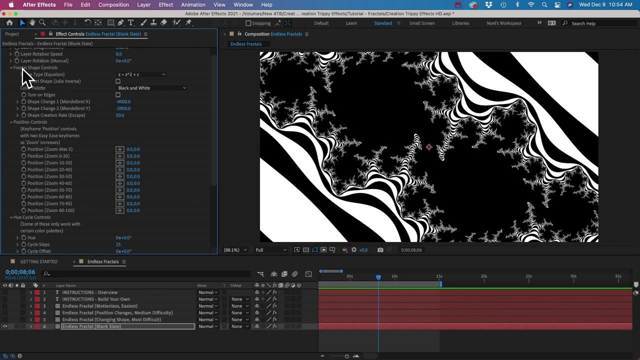 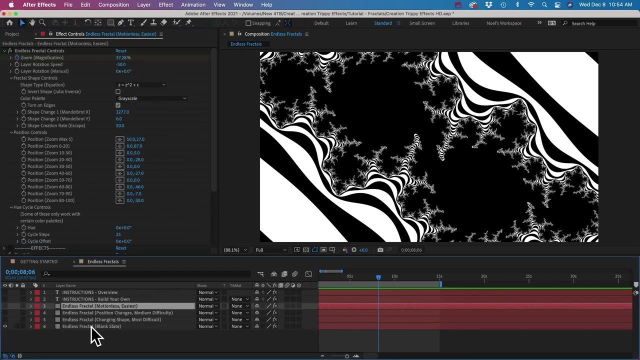 those later And you can see all the controls are divided into categories. So we've got these color controls at the bottom, and then we've got our position controls, and then these ones affect the shape of the pattern. So let me show you how to make one like this, the easiest kind. First of 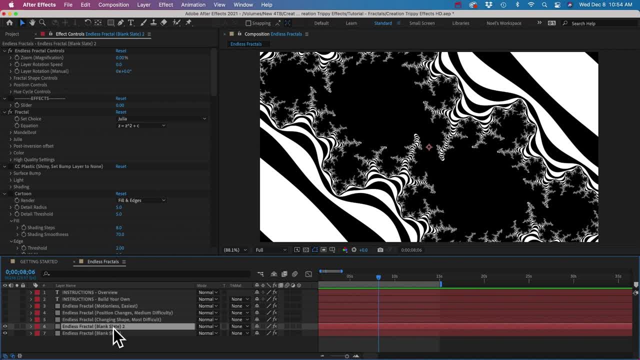 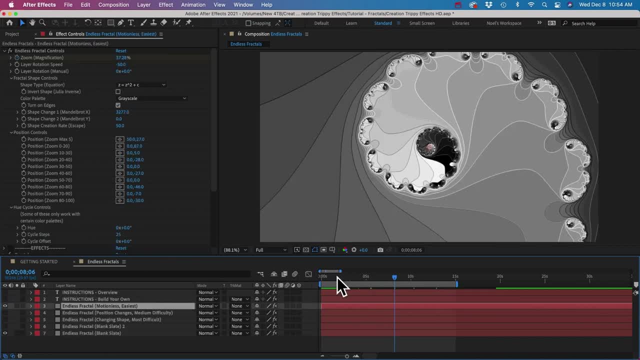 all, I'm going to duplicate this layer. So we have a backup of this layer and we're going to create a new one. I'll work on this one. Let me show you this one first and scrub through so you can see what's going on. It's just zooming in forever, And this one's the easiest because the 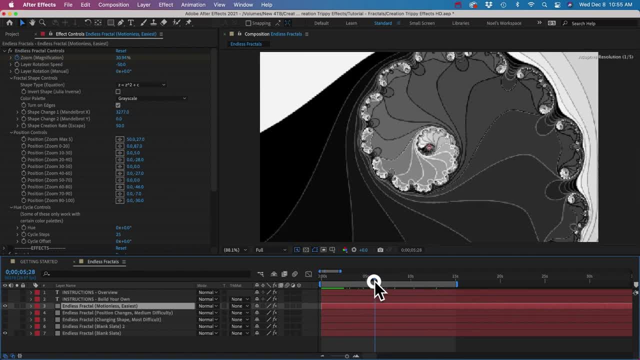 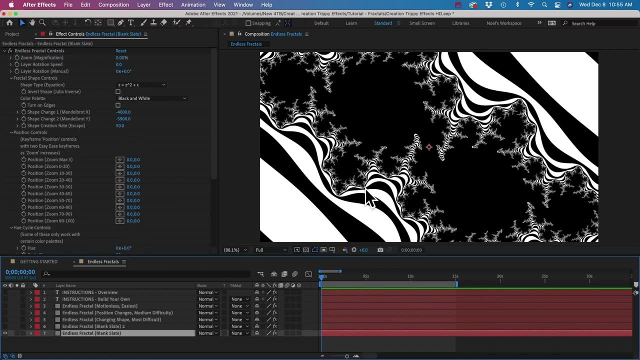 shape doesn't have any movement. It's not changing shape or position, It's just zooming in. So let's make one like that. The first thing you'll want to do is find a shape or pattern that you like, So you'll want to play with these shape controls and just try and create something that looks. 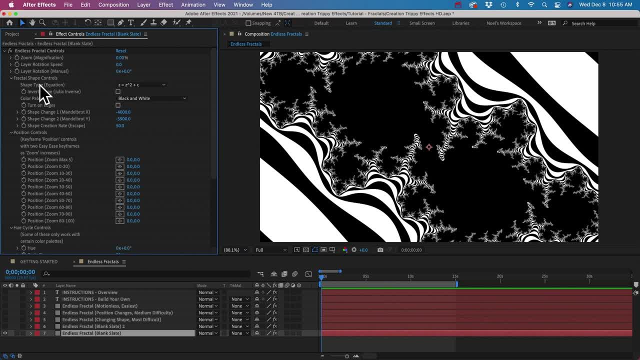 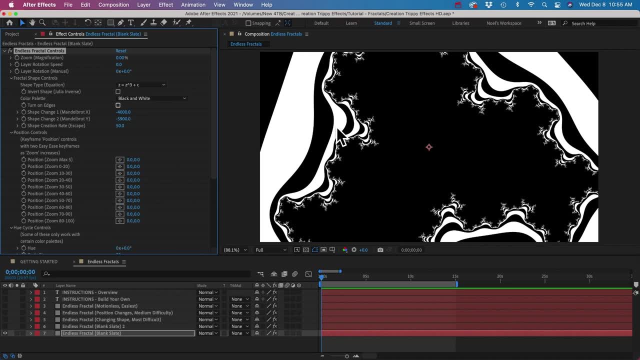 interesting. So with the shape type you can change the formula. And I should explain fractals. from what little I understand, they're just mathematically generated patterns, So they use some weird formula to create this pattern. They're basically vector-based designs, so they never lose resolution. So you 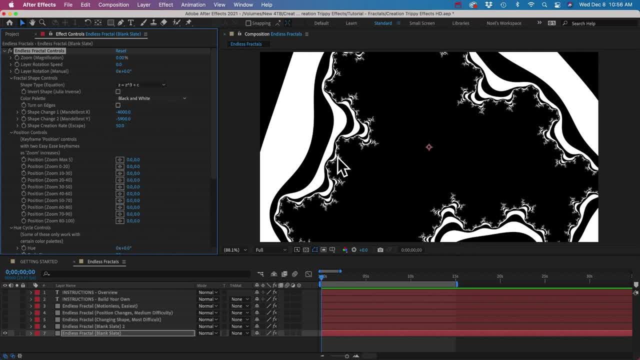 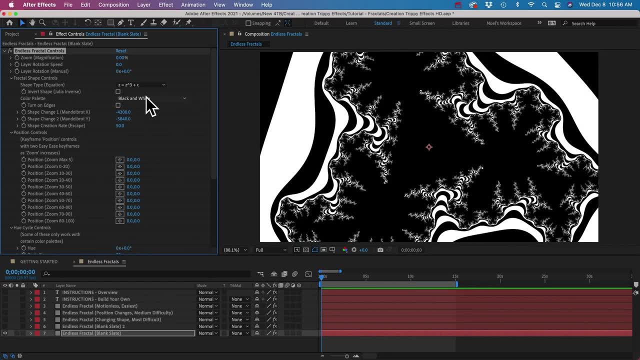 can just keep zooming in forever and the formula will generate new patterns And with these controls you can adjust the shape of it and you can choose a different color to call it. If you want, you can turn on the edges and give it kind of an outline. 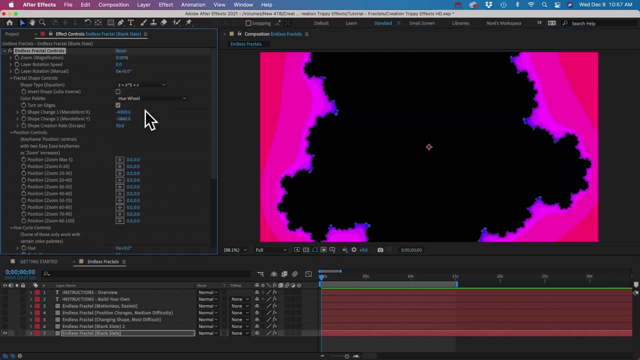 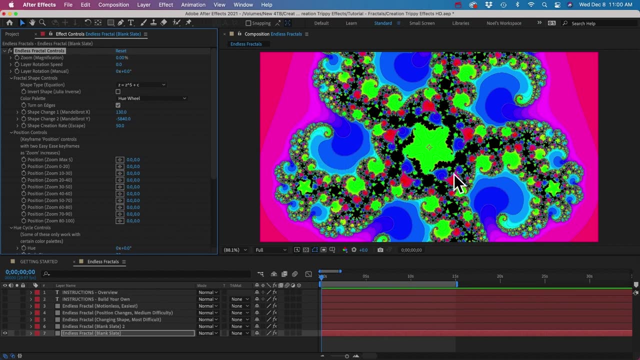 All right, I can work with this. So once you choose your shape, you're going to want to choose an area that you want to zoom in on, And then you can put that area right in the middle of the frame using this first position control. So it really doesn't matter, I'm just going to zoom in right here. So I 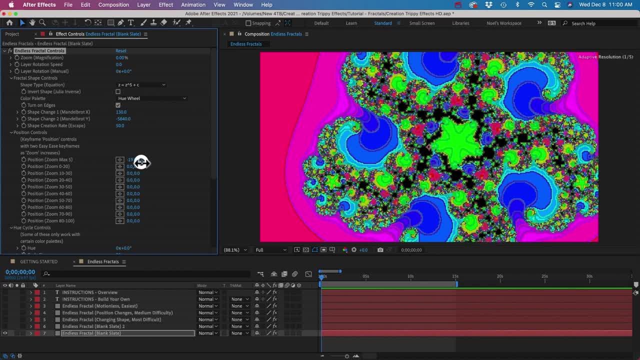 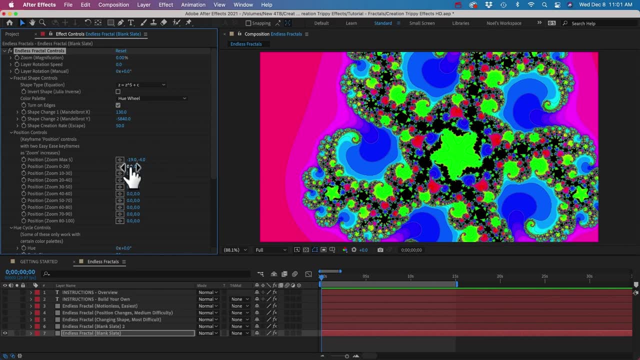 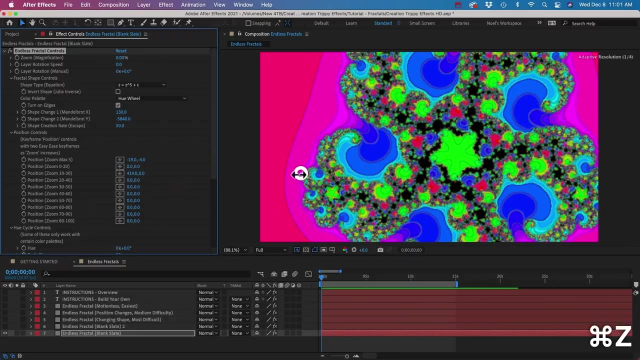 would use this first position control to move that kind of to the center. Now maybe you saw when I dragged this value, this moved pretty quickly. If I drag the second one, the second position value, it's not moving nearly as quickly. If I drag the third one, you don't even notice any movement. So all 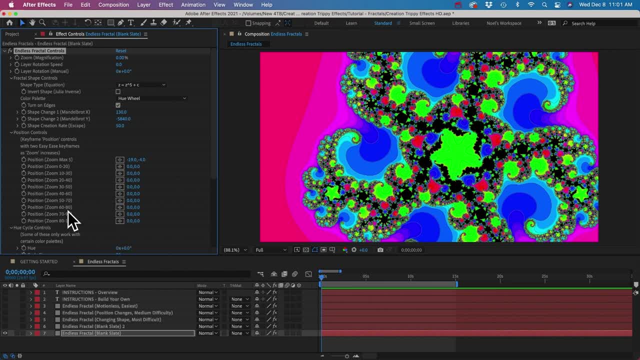 of these will change the position, but they're varying degrees of sensitivity And each one is intended to be used at a specific zoom value. So right up here at the top, we've got our zoom control, And if the zoom is set to 5% or 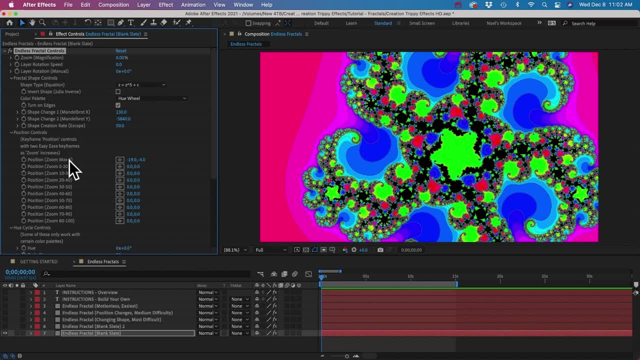 less. we would use this first control because it says zoom maximum 5.. If it's set anywhere from 0 to 20%, we would use the second control. If it's set from 10 to 30%, we would use this one, and so on. 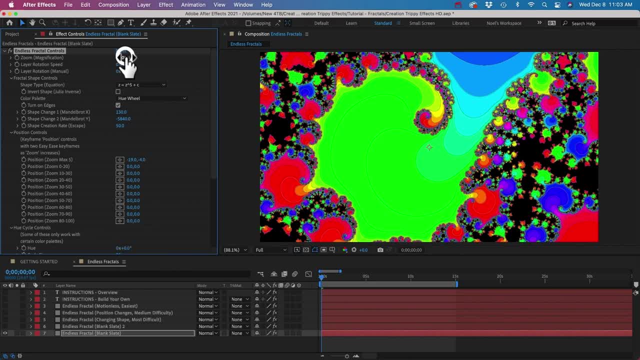 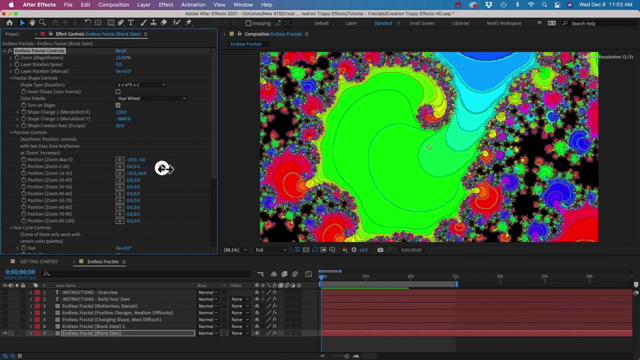 So now that this is kind of centered, let's zoom in a bit. All right, so I'm zoomed in a little bit at 12%, And now we can define a more precise area to zoom in on At 12%. I would use this control here. I like zooming in on spirals, And then I'll go a. 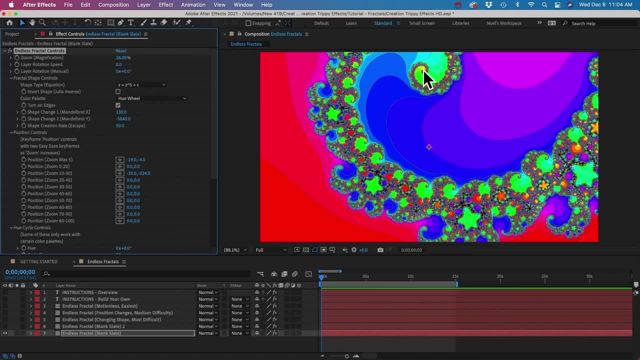 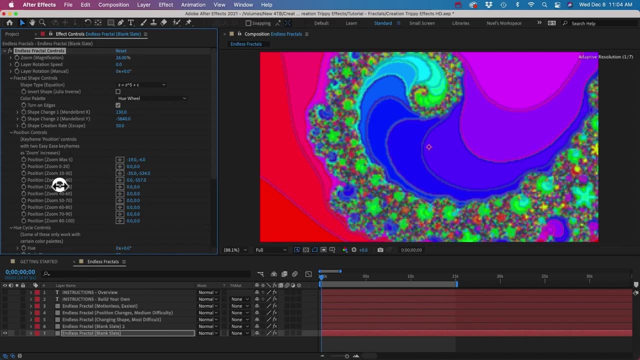 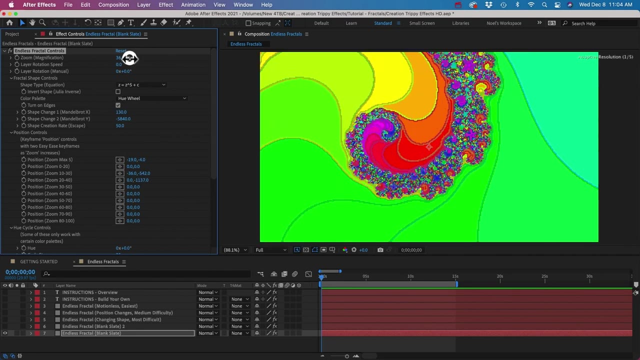 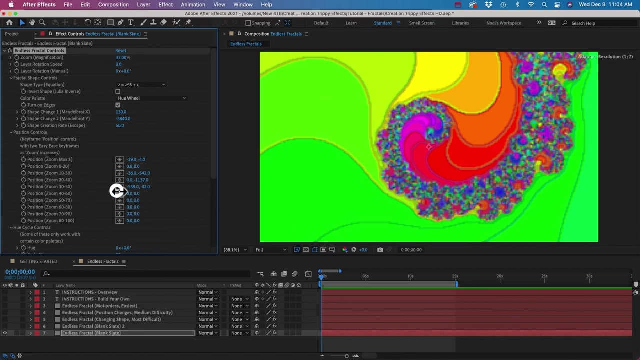 little bit closer And I'll just keep going in on that spiral. I'm at 26%, So I'll use this one here. I'll zoom in a little bit more And then we'll just keep doing that. I'll keep zooming in little by little. 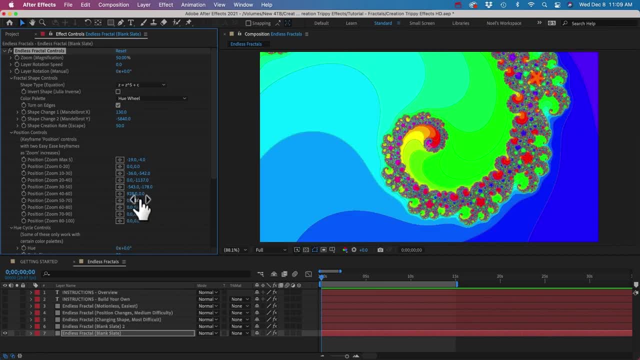 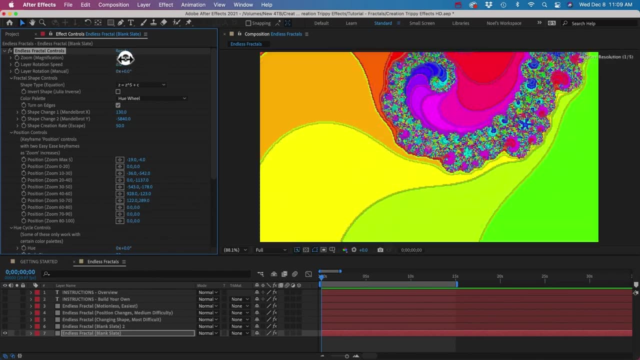 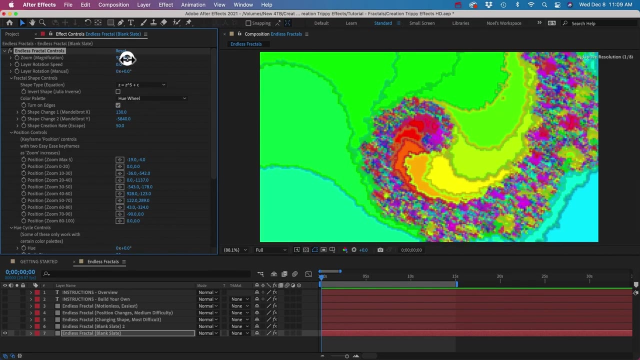 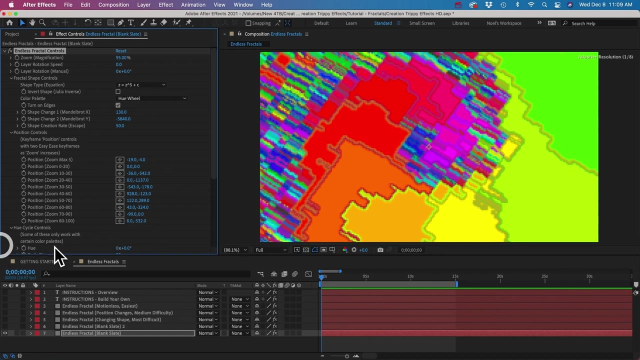 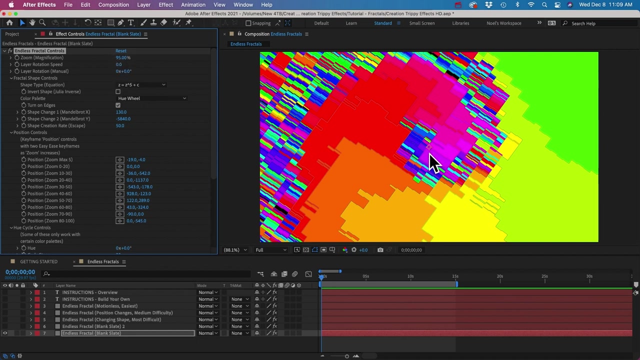 and then reposition it All right. As we near 100%, you'll notice that it starts to get kind of funky, So you do eventually start to lose resolution. Going all the way to 100% does provide quite a bit of zoom, But if you do need something that keeps going, or if you need it to loop, that should be. 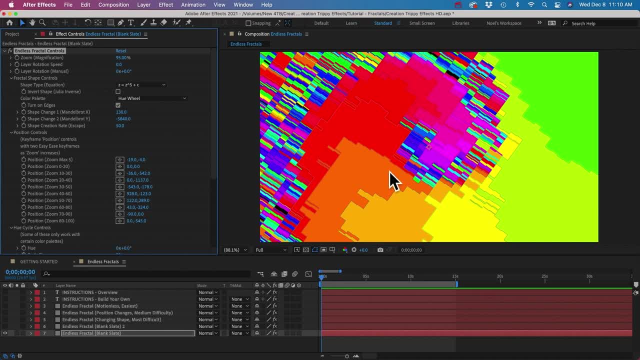 possible. You'll just need to make sure your animation looks similar to what you want it to look like. animation look similar on the first frame as it does on the last frame. It doesn't have to be exactly the same, just as long as it's the same general shape and position, And then you'll be. 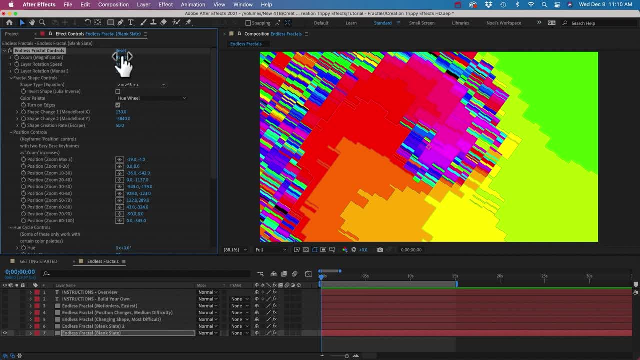 able to take that animation and fade the end of it into the beginning, And I show how to do that in another tutorial that I made a long time ago And I'm going to put a link in the description to that tutorial. So if you need a looping animation, you can check that out. All right, 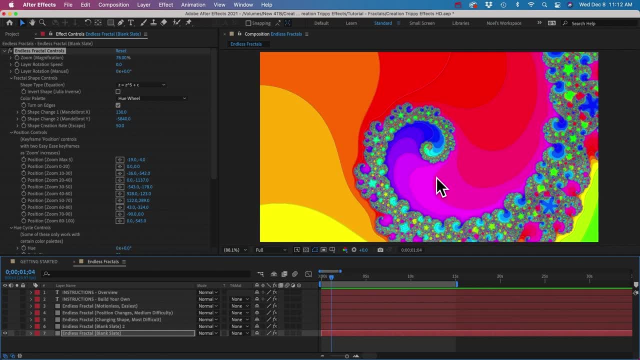 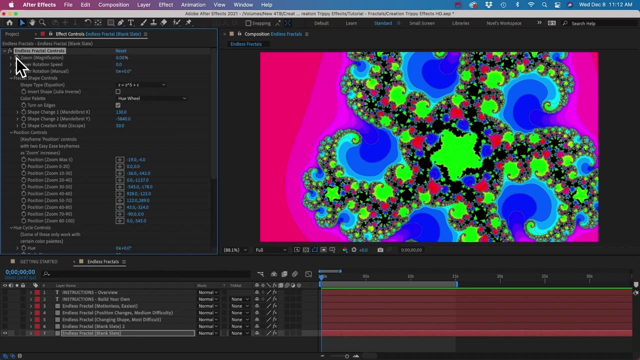 so this is positioned perfectly. All we have to do is animate the zoom control. So I'll go to the first frame and I'll set this to zero And I'll add a keyframe And let's say: we want this to go. 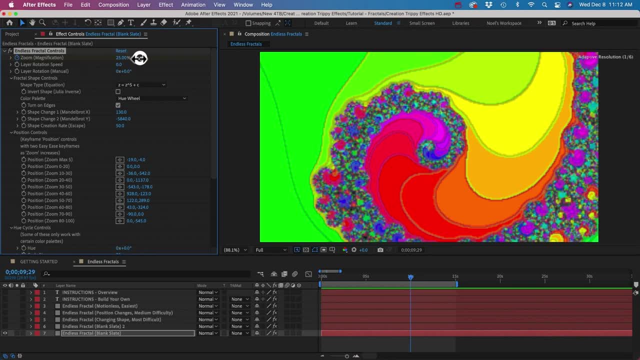 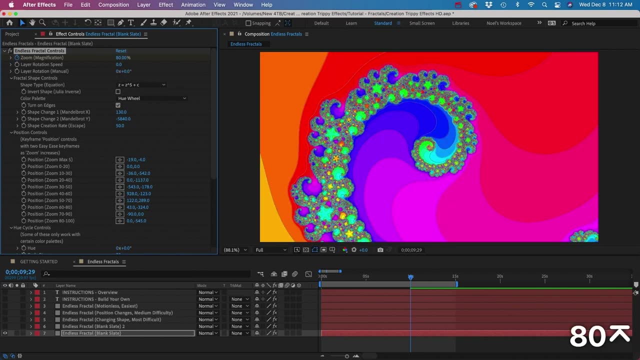 on for 10 seconds And I'll set this to. I'll do 90 or 80.. All right, if I hit the U key, you can see those two keyframes. These are linear keyframes, the little diamond ones. That means that the pace is constant throughout the whole animation. 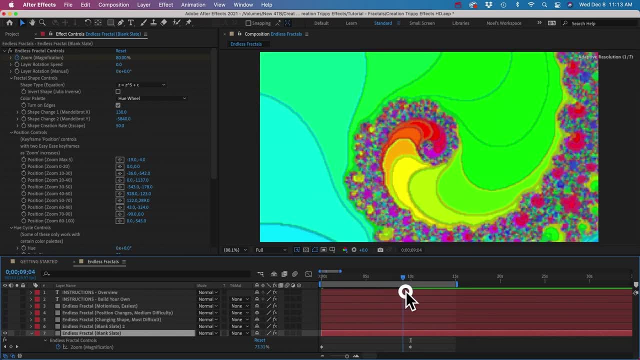 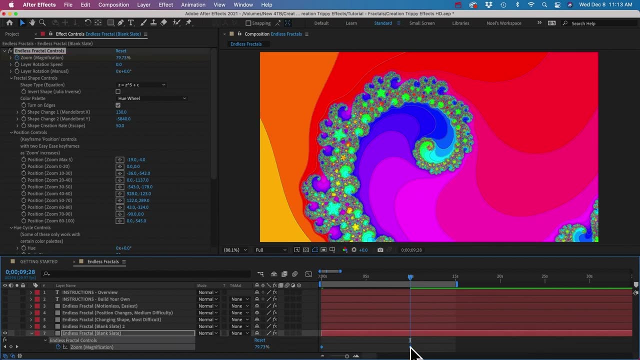 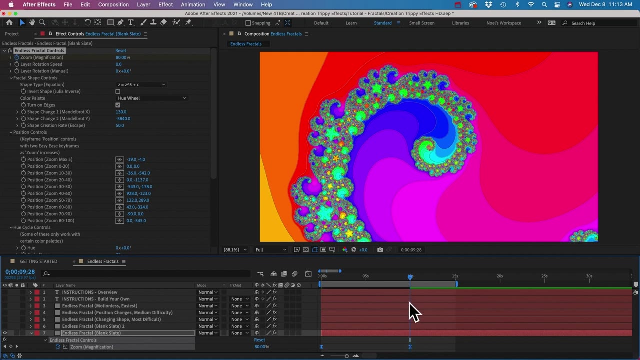 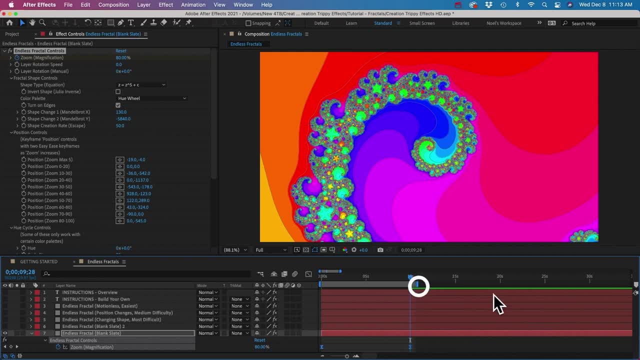 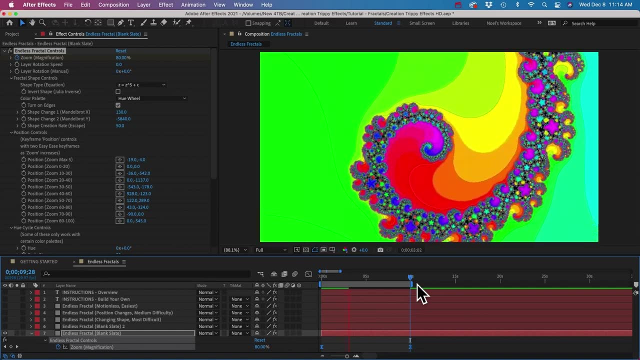 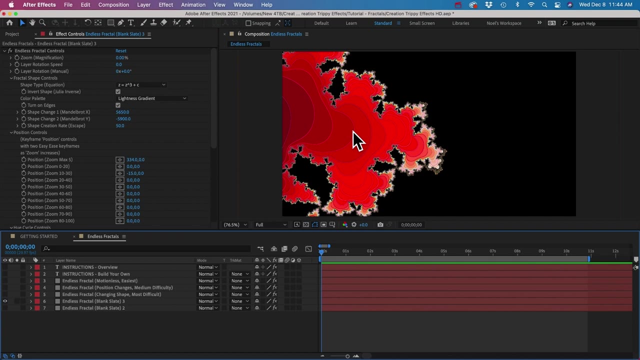 and do that. right here I'm going to set the out point. You can do that with a shortcut, That's the N key, And let's do a quick preview. All right, let's create an animation like the second example, And I've already got a pattern here that I made, So for this one we need to animate our 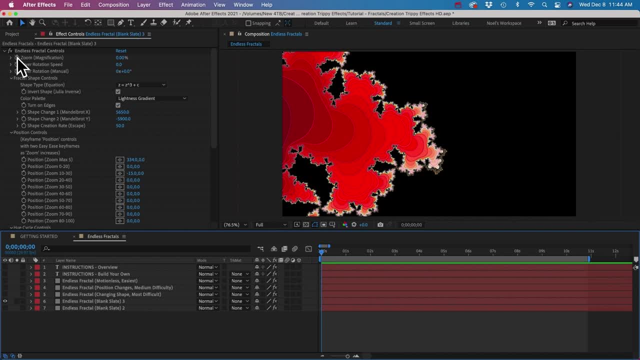 zoom control first. So I'll go ahead and add a keyframe for that at frame zero And I'll go forward And let's do 10 seconds again And I'll set this to 80.. So we can see it's just zooming in on this. 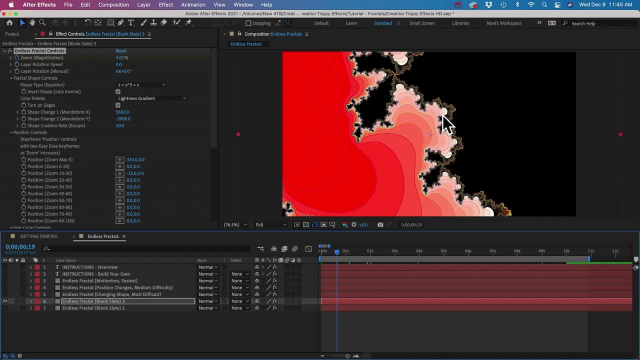 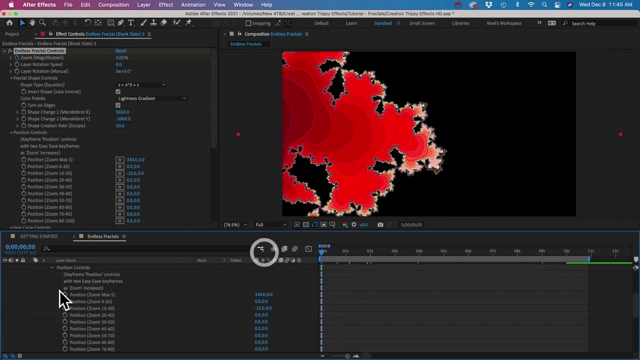 blank area of the pattern. So we want to add keyframes to these position controls to make it zoom in on new, more interesting areas. So let me expand this layer so that we can see our position controls down here. All right, so we can just add a keyframe here for the first one And for this. 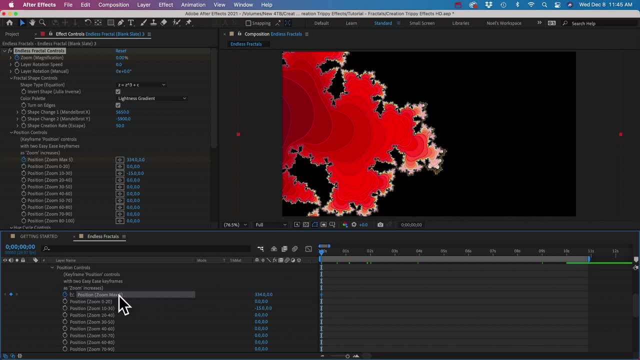 position control. you can see that it's just zooming in on this blank area of the pattern And you can see that it's meant to be used for up to 5% zoom. So I'll scroll up so we can see our zoom. 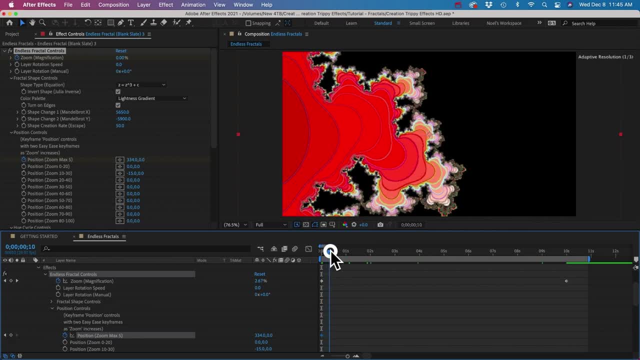 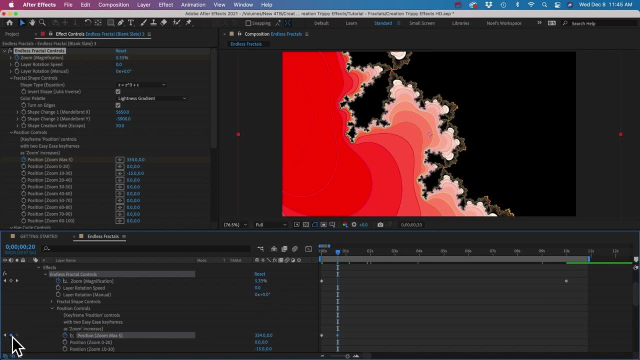 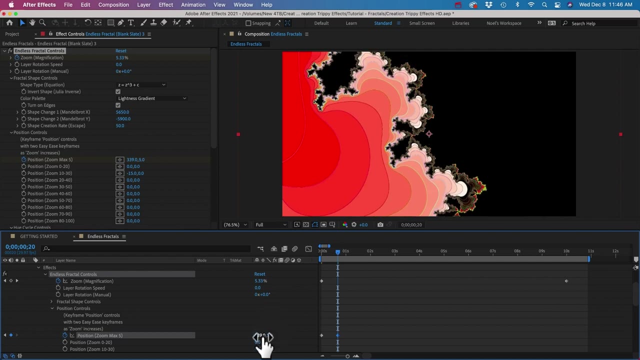 value And I'll just scrub forward a little bit until we get to about 5%, And then I can add my second keyframe, And you don't have to add it that way, You can just change the value to wherever you want and it'll automatically add that keyframe. So you see how fast it's moving when I 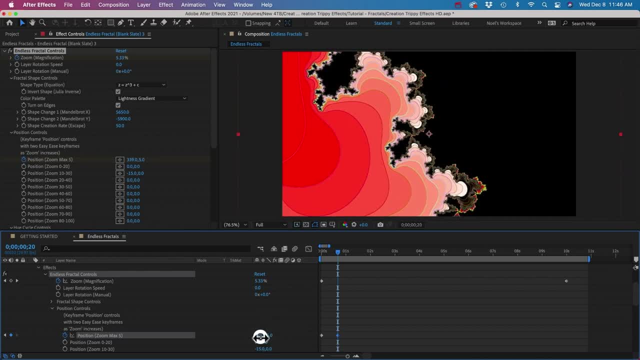 drag this value. So here's a tip: If you hold down the command keyframe, you'll see that it's going to change the value. So if you hold down the command or control key on your keyboard and then drag the value, it'll reduce the amount that it changes as you drag it, And the opposite of 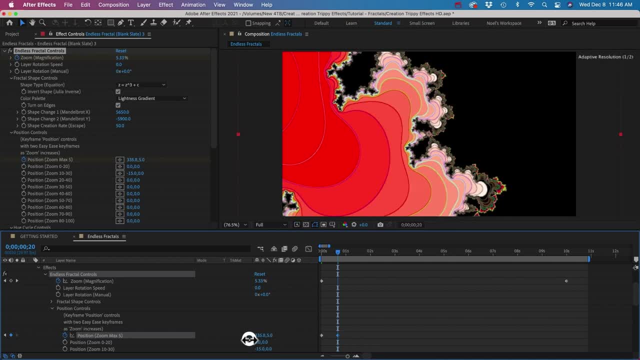 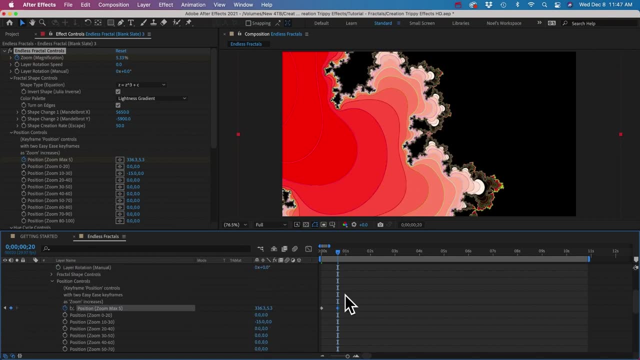 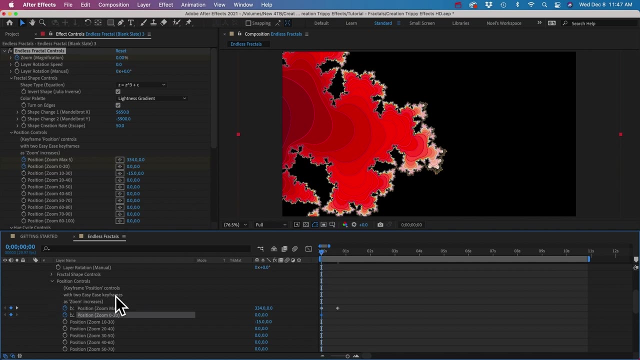 that if your value is changing too slowly, you can hold down the shift key and then drag, and that'll increase the amount that the value changes. Anyway, we've got our two keyframes. Let's do the next position: control This one. I'll start on frame zero two, And this goes from zero to 20.. 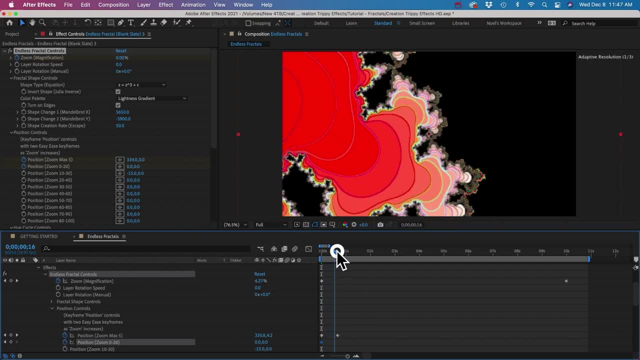 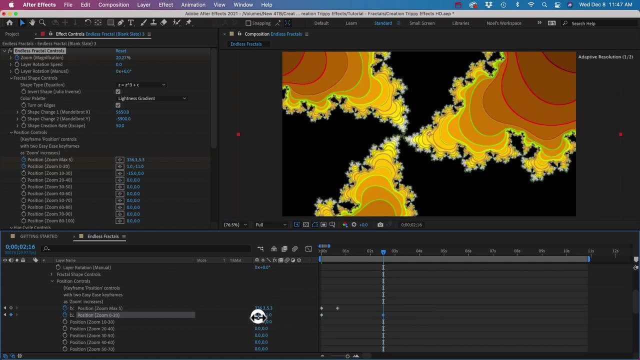 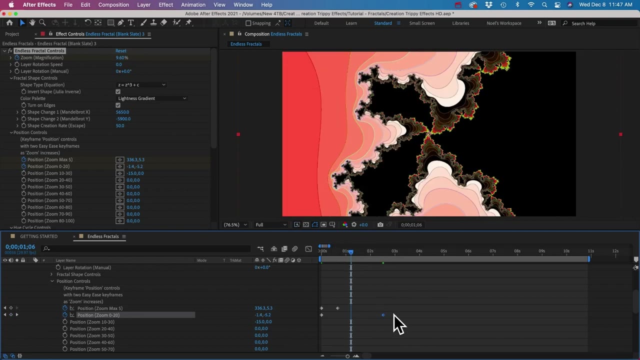 Let me make it so we can see our zoom, And I'll go forward until the zoom is at 20%, And we'll position this to wherever we want. All right, let's do the next one, And rather than just starting right here and adding a keyframe for the next control, let's go back about halfway in between. 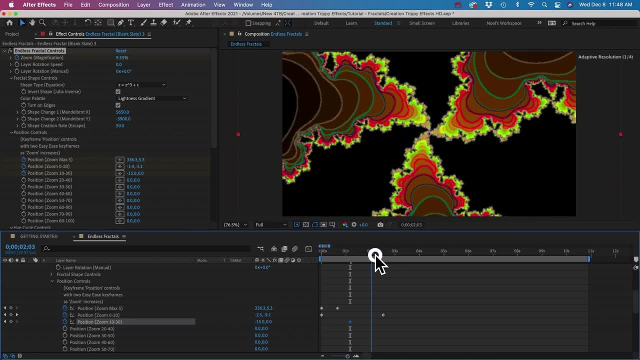 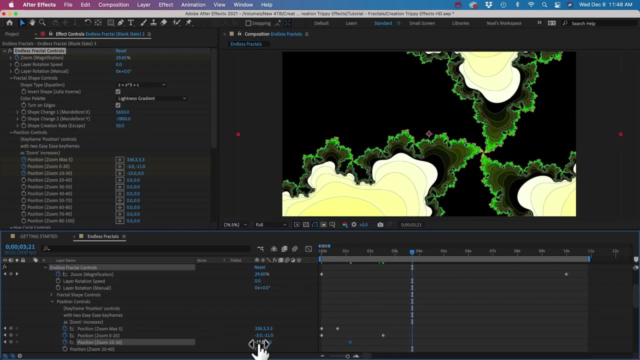 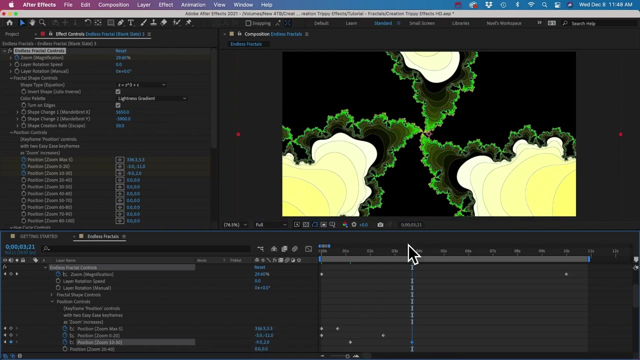 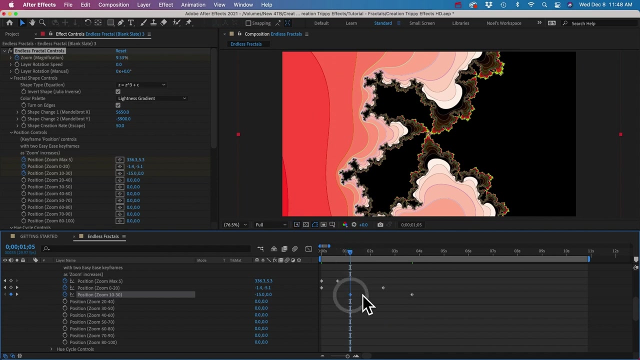 the last pair of keyframes we made So right around here And we're going to go to about 30% and we'll change the position And I haven't really moved it much, So let's do that with the next one. And the reason I went back to here is because we want each pair of keyframes to overlap each. 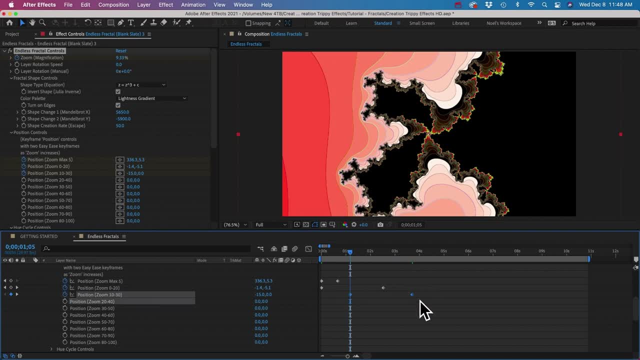 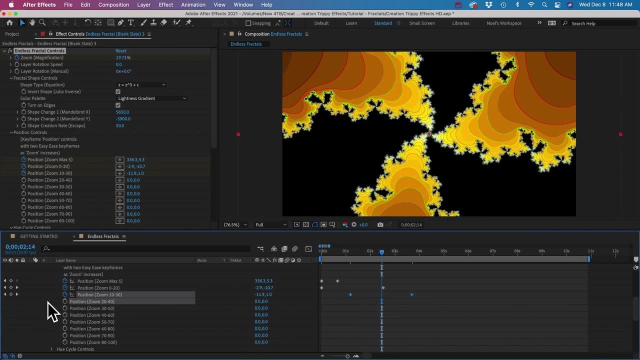 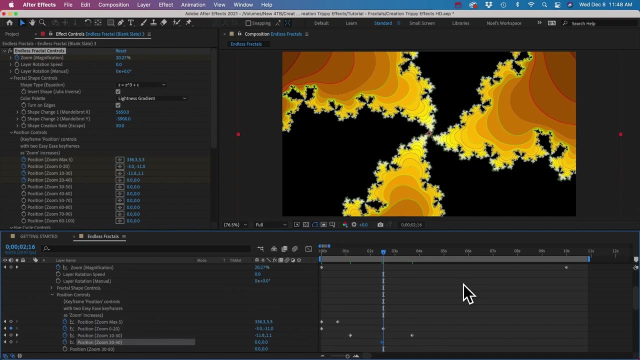 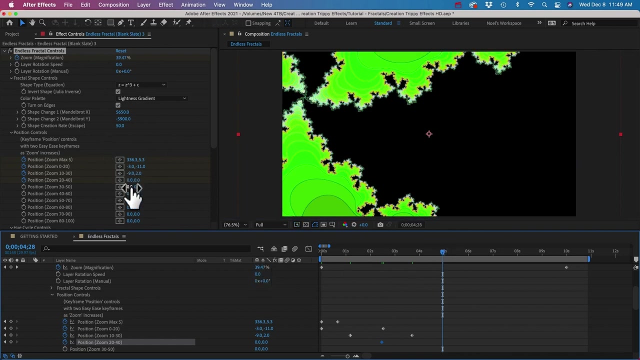 other, And that's going to make the movement much more smoother in the end. So for the next control, we'll go halfway between these two keyframes. Let's add a keyframe there. We'll go forward to 40%. Okay, we're at 40% about And let's move somewhere new. 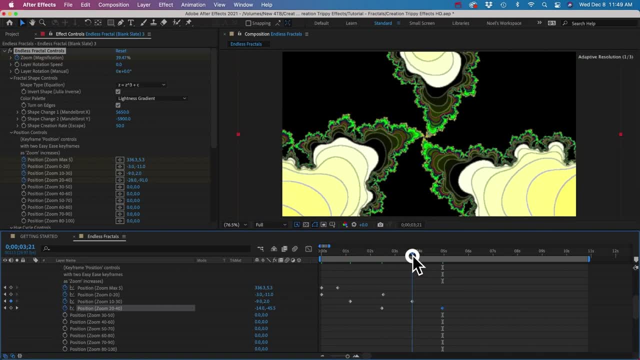 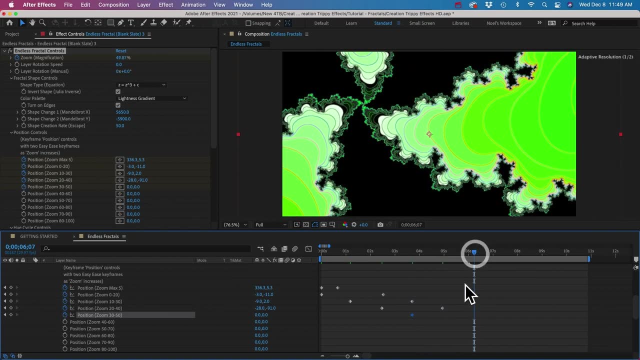 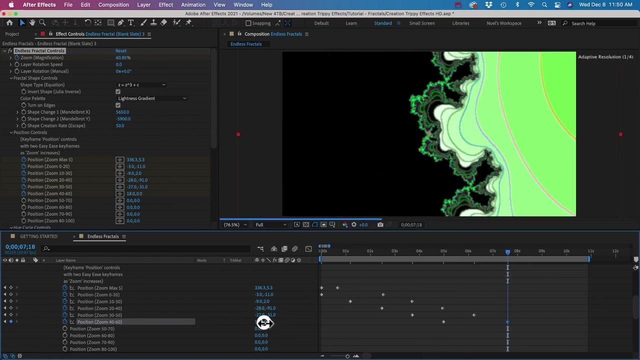 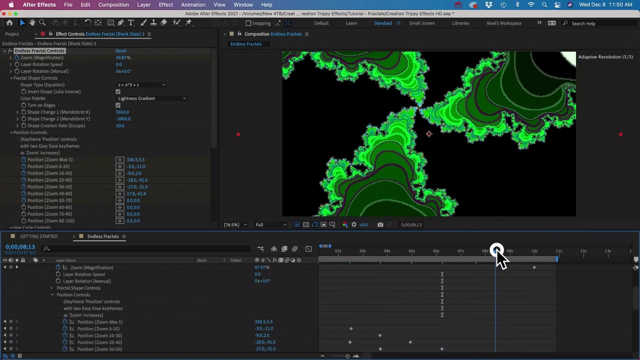 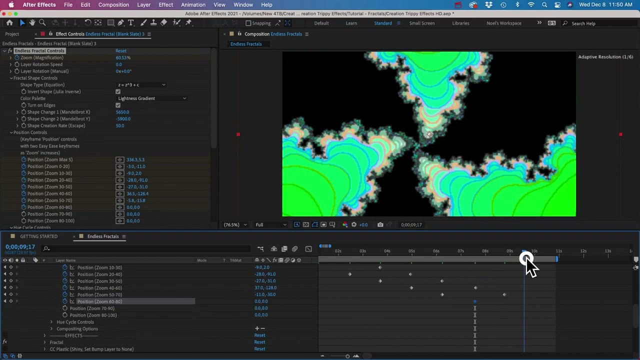 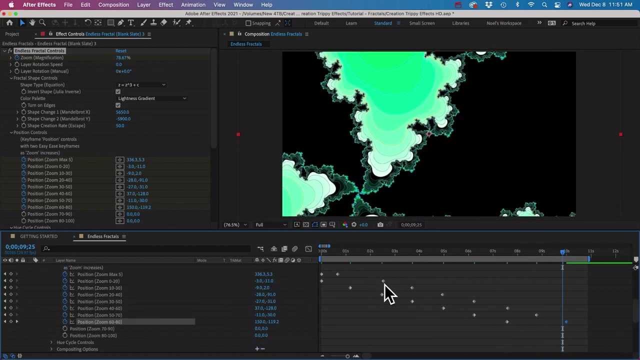 I'll be right there. We'll just keep doing that all the way to the last position control. I can kind of guess where the next keyframe is going to be. They're all about two seconds apart from each other, All right, so I reached the end of my zoom. We talked about linear keyframes. 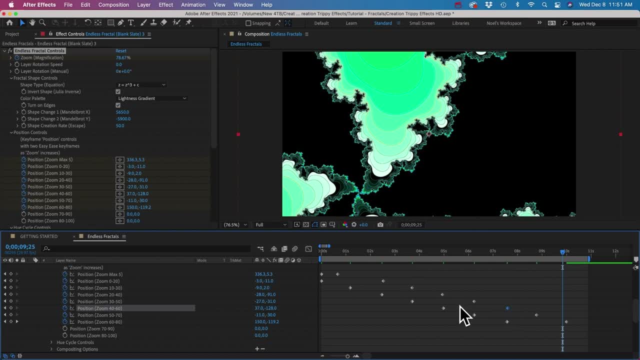 these diamond ones, which means all of the movements are at a constant pace And it's not going to look very good. It's going to look kind of jerky To make them smoother. we want to select all of them and make them easy. easy keyframes, And let's see what we got. 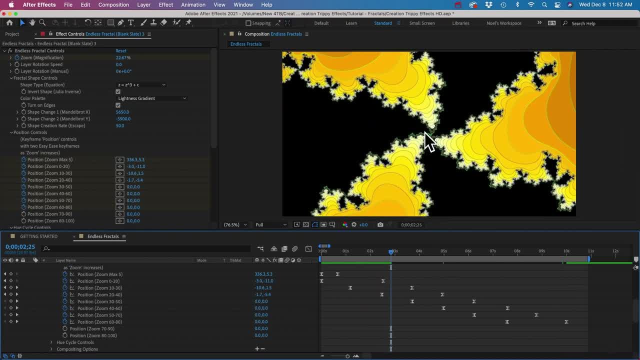 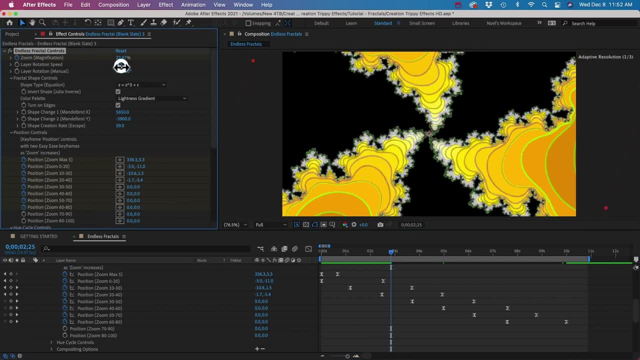 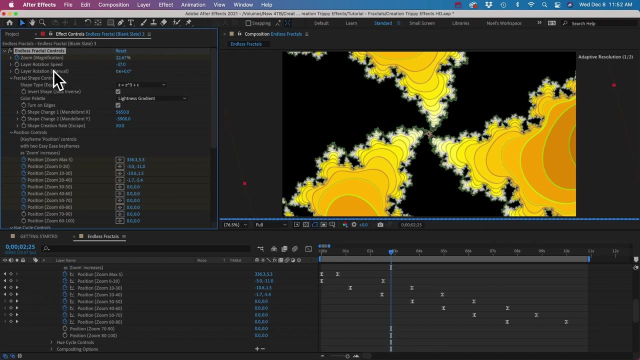 And I didn't add any rotation of this, but I think it could use some. There's a control up here that lets you set the layer rotation speed. Use a positive number to make it rotate clockwise, or negative to go counterclockwise, Or, if you want to just keyframe it manually, you can use this. 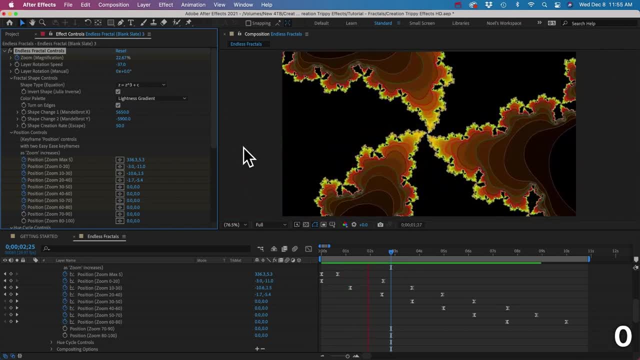 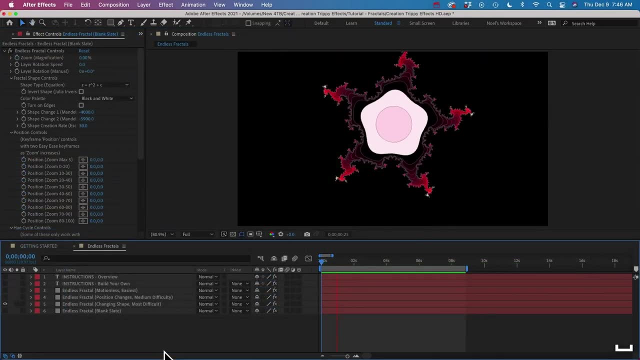 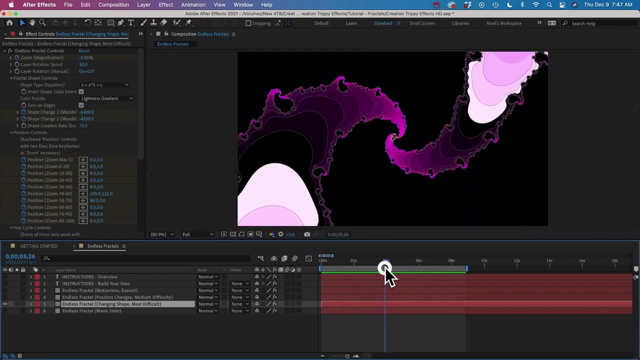 manual control. Okay, let's take a look at this third example. It's similar to the one before, but it's a little more difficult, because you can see the pattern is changing shape as we're zooming in. The reason that's so hard is because when it changes shape, all the different elements are moving around. 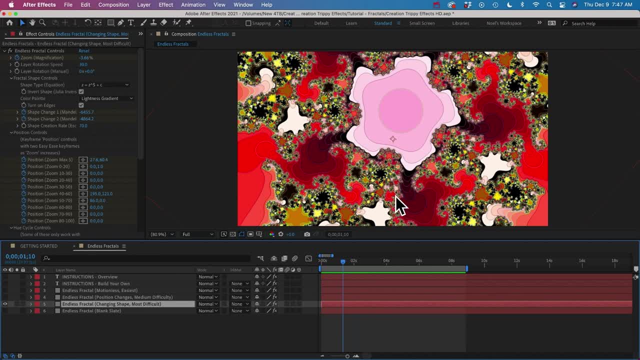 So that makes it really hard to zoom in on them, And for that reason you really shouldn't have the shape change once you pass a certain zoom value, Because if you're zoomed way in and the pattern is moving, it's just going to be too hard. 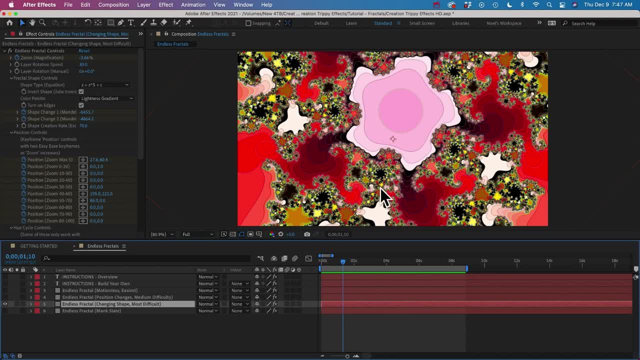 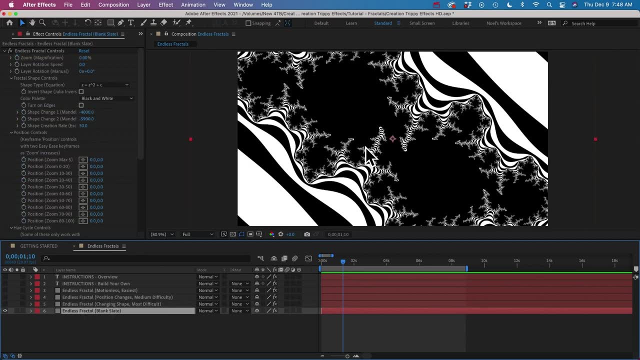 to keep an area in the frame. So there's probably lots of different ways of doing this, but here's what I would do. Let's go to our blank slate And, just like before, you would find a pattern you like. first I'll just go with this default pattern. 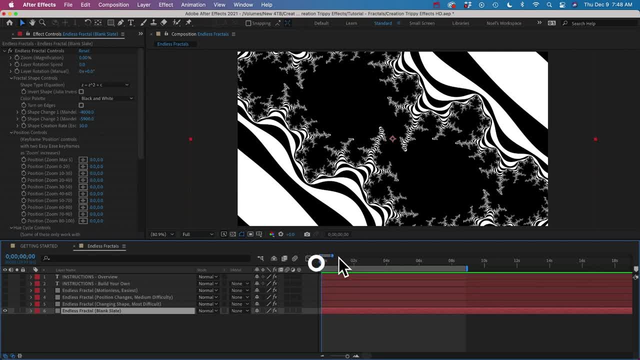 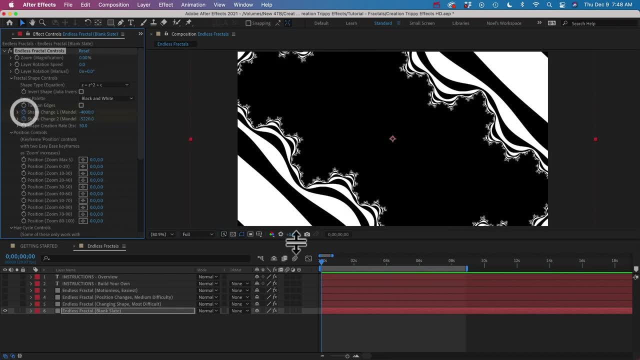 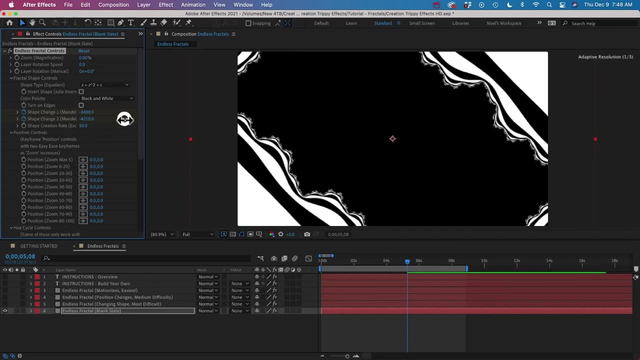 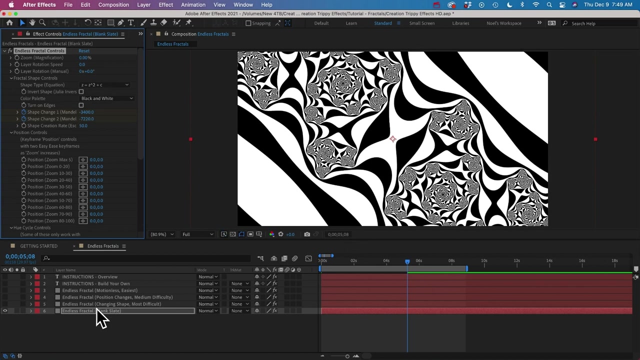 And then I would add my shape, change keyframes first. So that's these two controls. You can have it start like this, Then I'll select that And then I'll go forward about five seconds and change it into something more interesting. Let's look at those keyframes By five seconds into this animation. 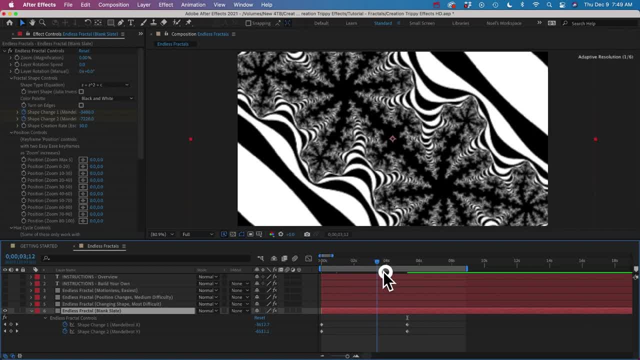 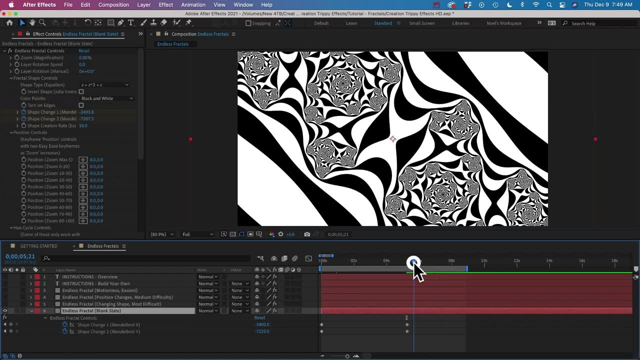 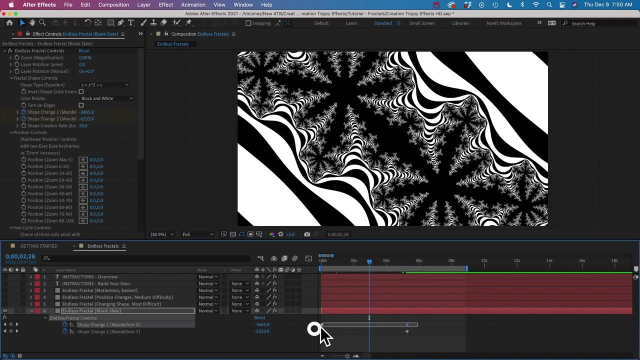 we're gonna be pretty far zoomed in, So even the slightest pattern change could make stuff just fly off the frame. So I want this pattern change movement to slow way down as it reaches this five second mark. So I can do the easy ease. 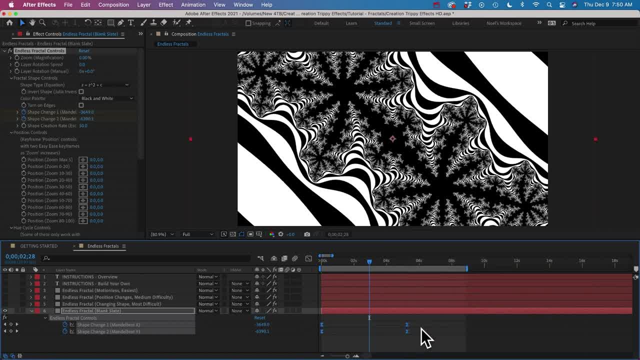 I can select these and go to keyframe assistant and choose easy ease, But that might not be enough, So I'm going to use the graph editor. That's this little button here. Let me make this bigger. I'll just try to explain briefly how this works. 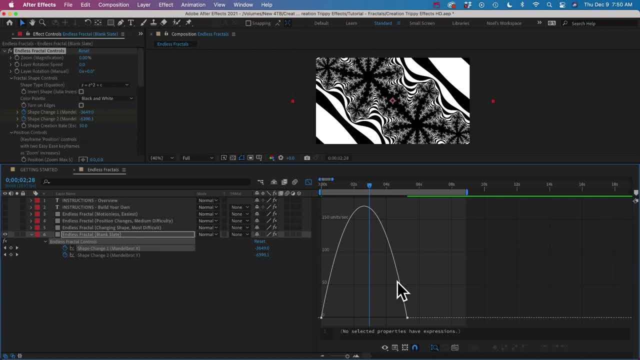 If you select a control with keyframes, you can see this line which represents the movement. You can see we've got it on the speed graph right now. So this line represents the speed at which this value changes. So you can see, here it starts at zero pixels per second because we've got these as easy ease keyframes. 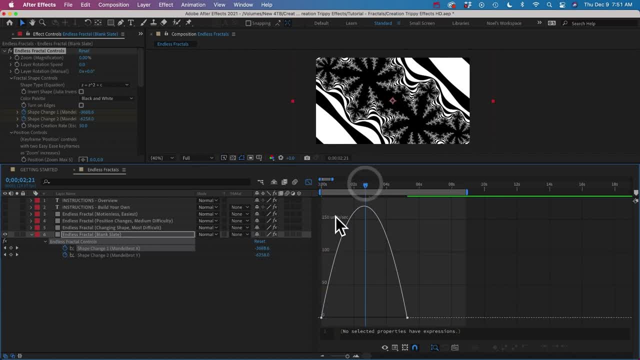 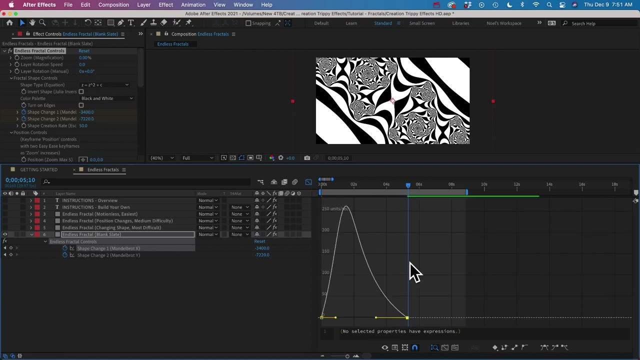 So it starts out slow and then it gets faster, And here in the middle it gets. It gets up to over 150 pixels per second And then it slows back down. But we can make it slow down even more if we select this little point there and then adjust the handle. 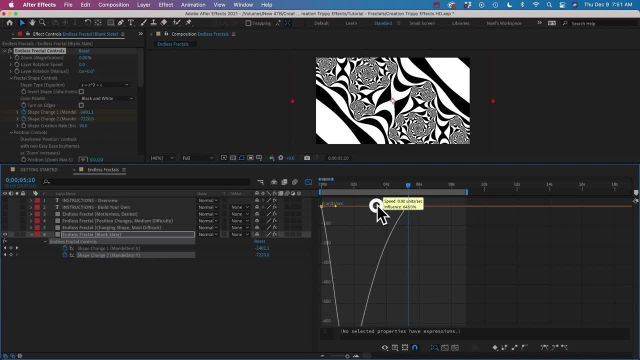 And we'll do that for the other one too. It doesn't look like I did much, but that makes a big difference. All right, And then, before I even keyframe the zoom, I think I'll move this into place while everything fits in the frame. 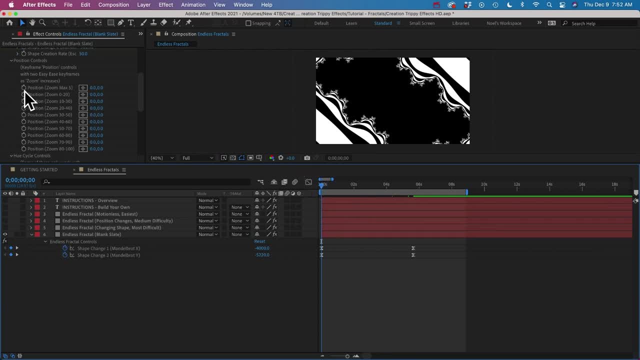 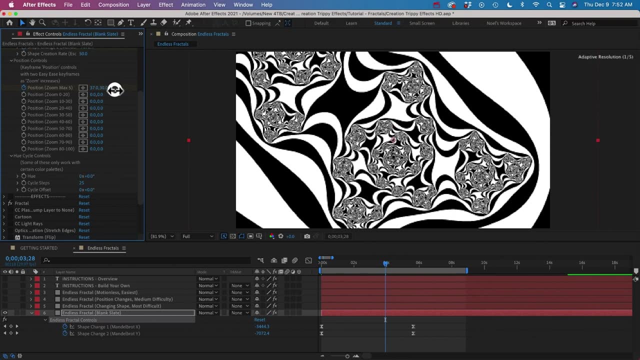 So Let's add our first position keyframe at frame zero and then go forward a little bit And we'll just move this to this spiral. Oh, and I'm choosing this spiral here because Let me get rid of those position keyframes. 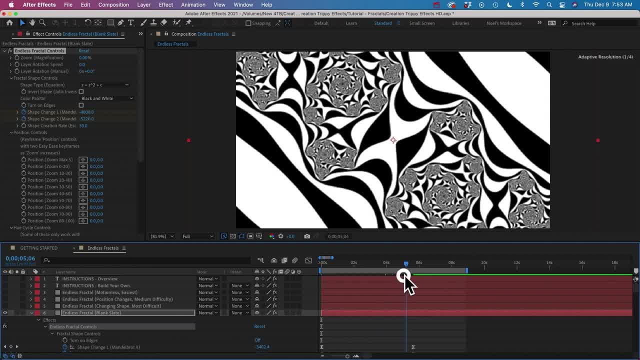 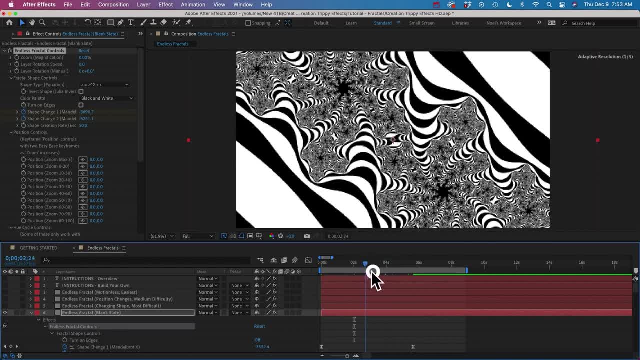 All right, If I scrub through, you can see the pattern changing shape. Some areas are moving around a lot, but you'll notice that right in the middle of this spiral It's pretty stationary, So I'm thinking that might be the easiest place to zoom in on. 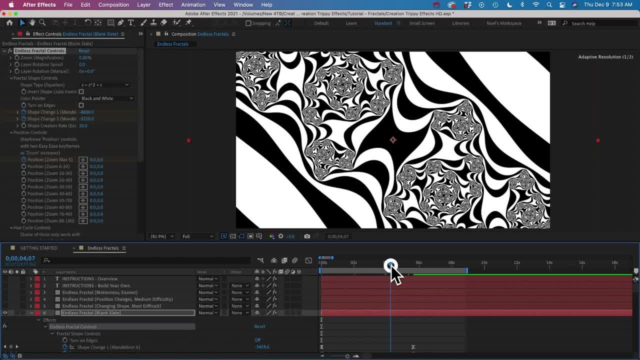 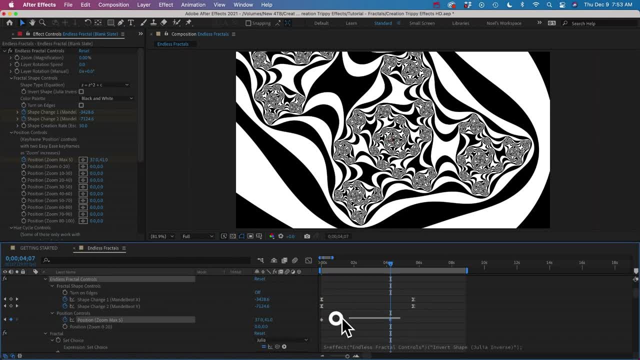 All right, So I'll add my first keyframe and then go forward a little bit and then move that area to the center And I'll make these EZEs as well, And I'll slow down that last keyframe in the graph editor. 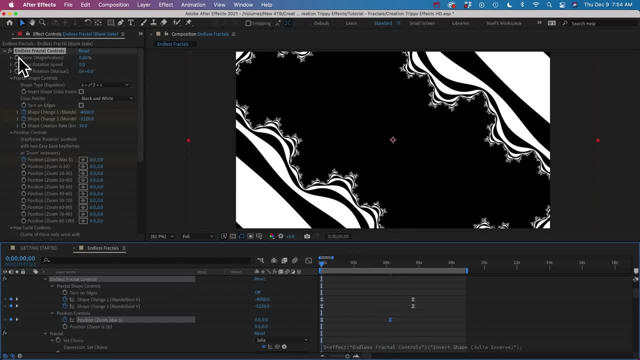 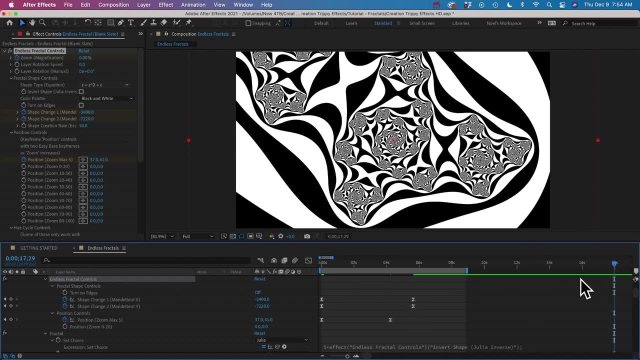 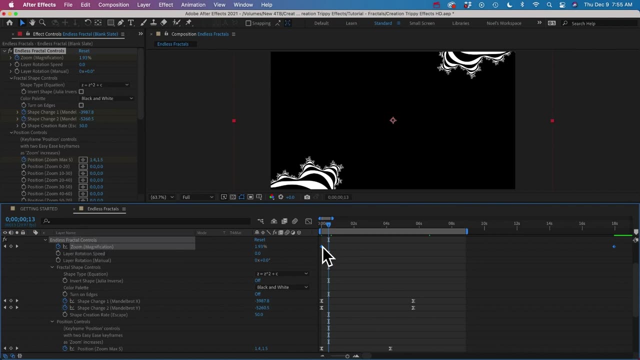 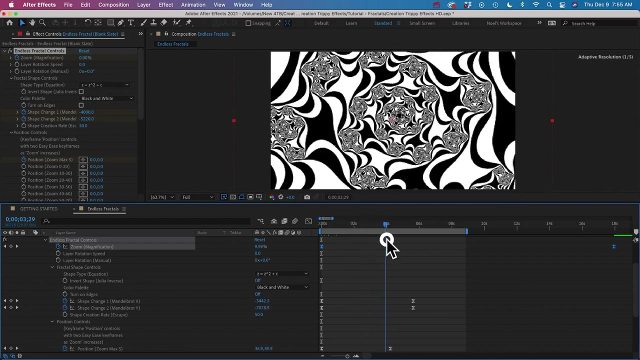 And now we can try adding some zoom keyframes. So So the zoom should last much longer than these shape change keyframes, And let's make these EZEs. Okay, let me see what that looks like. So that's pretty good. 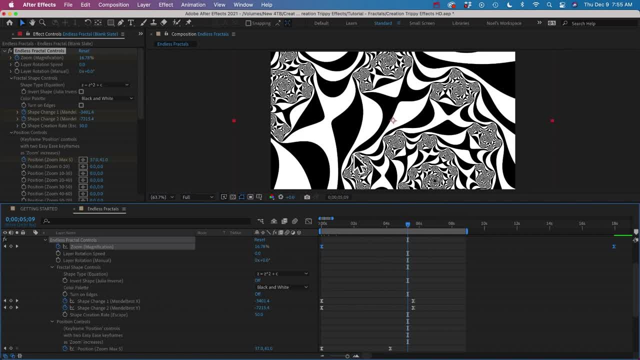 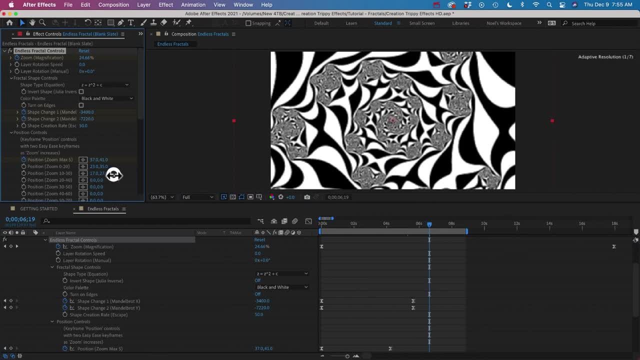 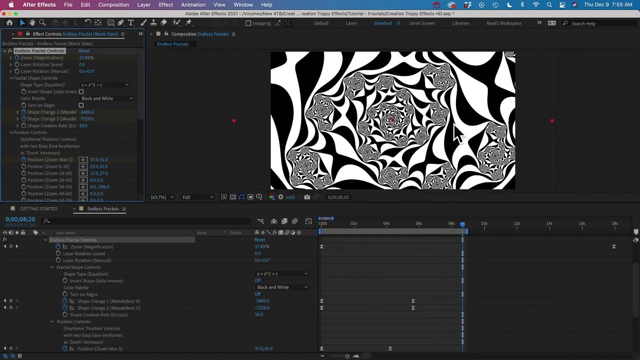 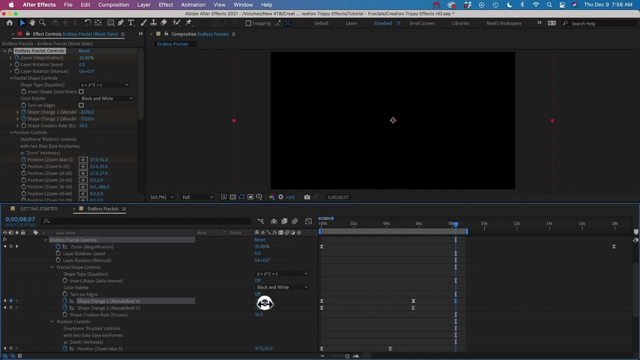 We want to fine-tune that position. So once you've passed your shape, change keyframes. it's just like before. You can zoom in on certain areas if you want, But you'll notice now that we're zoomed in. if I try adjusting these keyframes even a tiny bit, it just messes it all up. 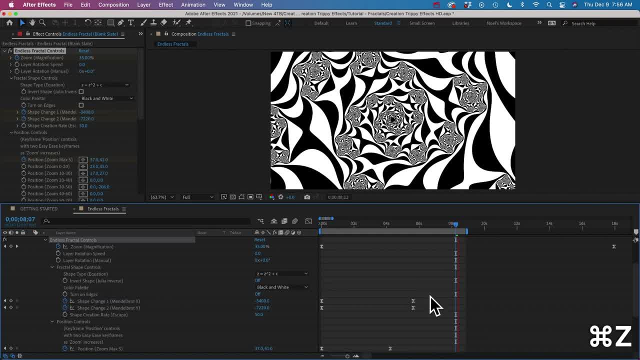 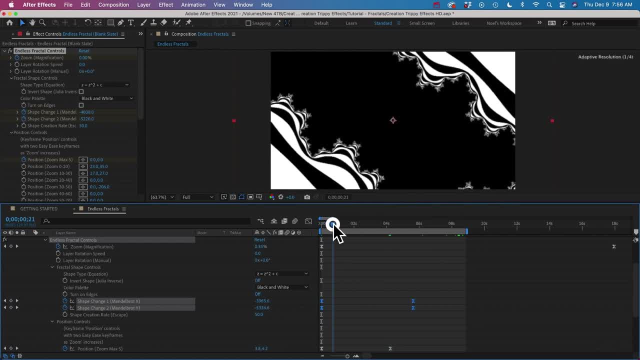 So just be careful with that. Make sure that your changes happen in the beginning of the animation. So you're kind of limited there, but I think it does add something cool to it when it's changing shape like this at the beginning of the animation. 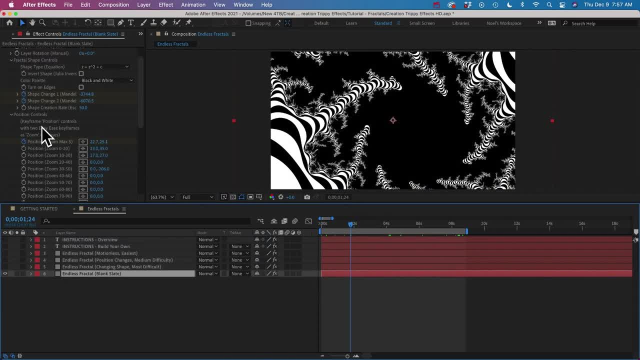 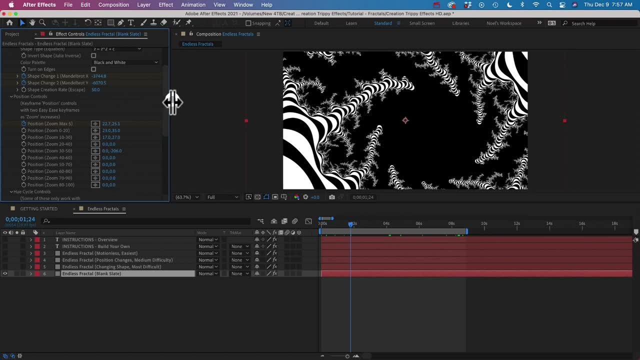 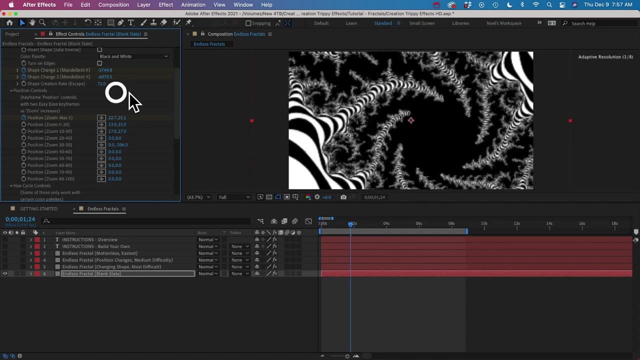 All right, let me show you a few other things we didn't talk about. There's a lot of opportunity to be creative here. I think You can keyframe some of these other controls, like this creation rate, And when you mess with that it affects the reach of the pattern. 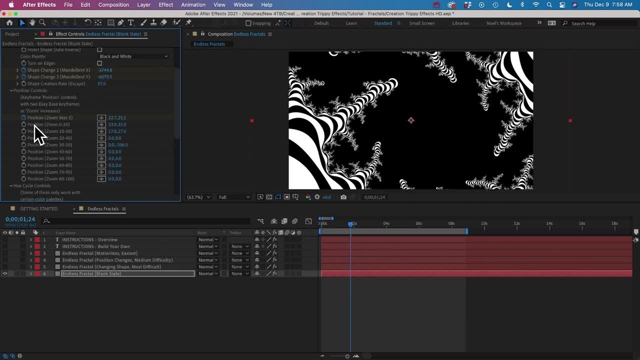 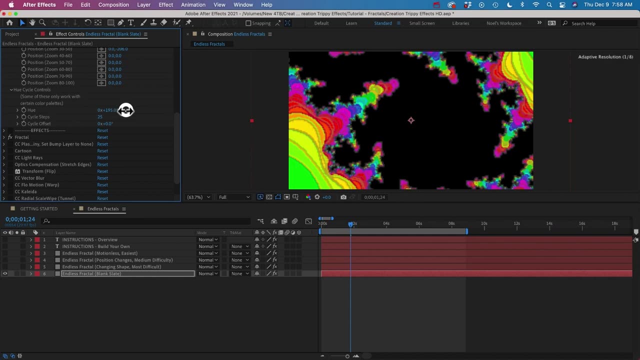 So it adds more detail. Further down, we've got some color controls, but some of these only work on certain color palettes. Like, if you change the hue right now, it doesn't do anything. But if you change the color palette to something with color, like hue wheel, now you can shift the hue and you can cycle the colors.